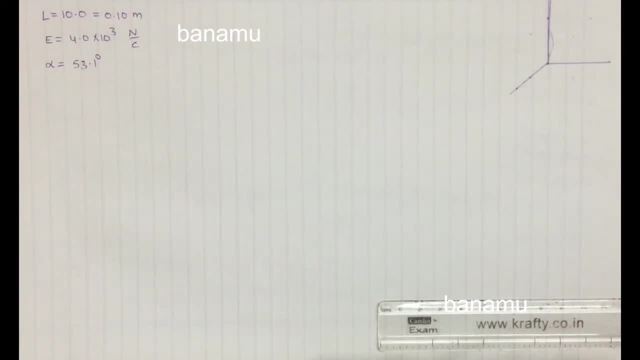 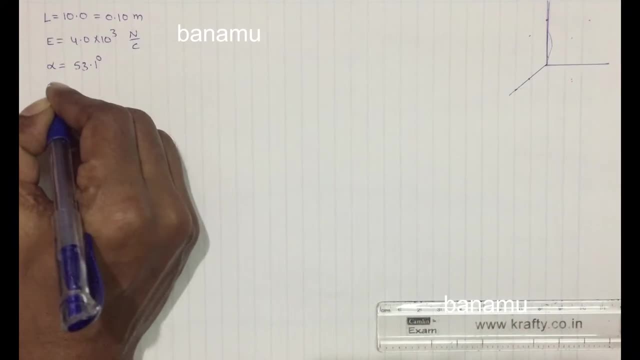 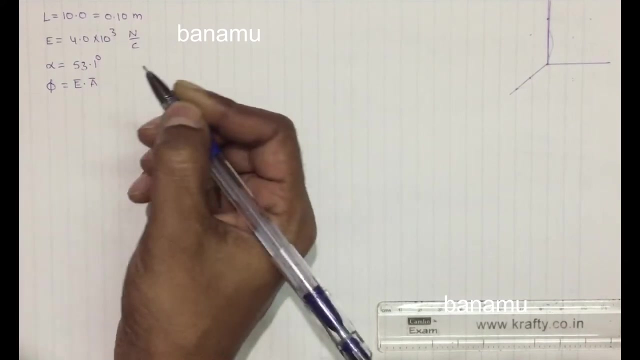 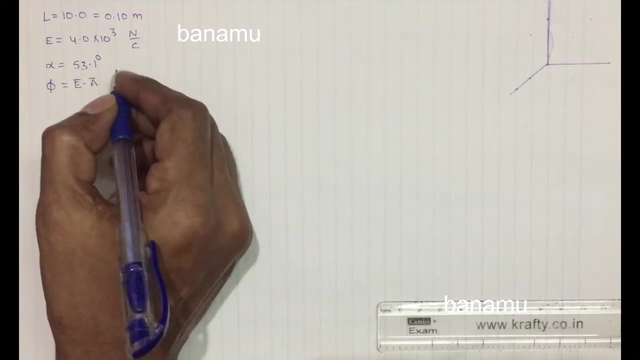 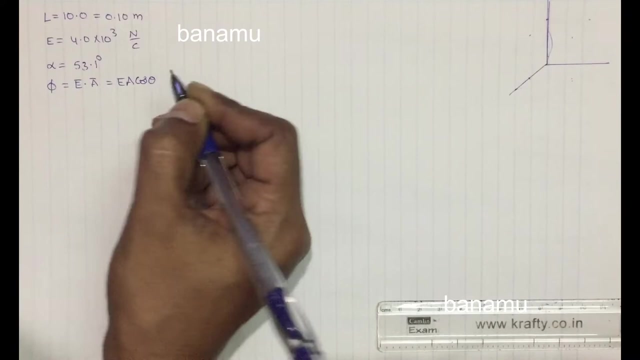 You can draw the, the electric flux through the each faces of the cube. The electric flux phi is equal to the electric flux phi is equal to e, e bar, dot, a bar, where e bar is the electric field and a bar is the area of the vector. that is equal to e a cos theta. 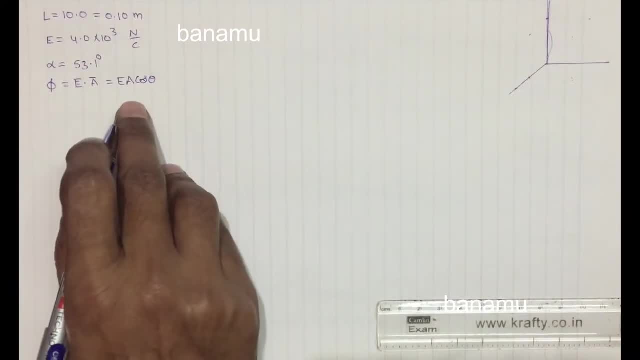 The electric flux phi is equal to the electric flux phi is equal to e a cos theta. The electric flux phi is equal to e a cos theta. Where theta is the angle between the electric field and area unit normal vector. Where theta is the angle between the electric field and area unit normal vector. 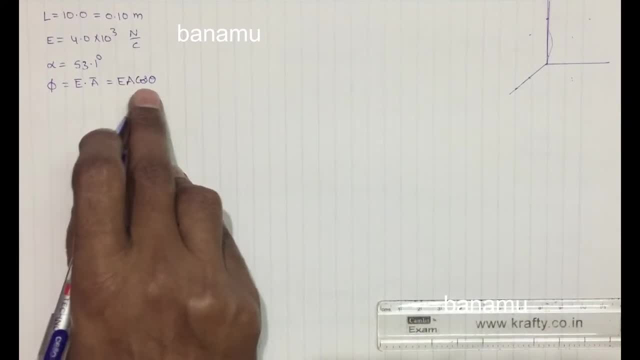 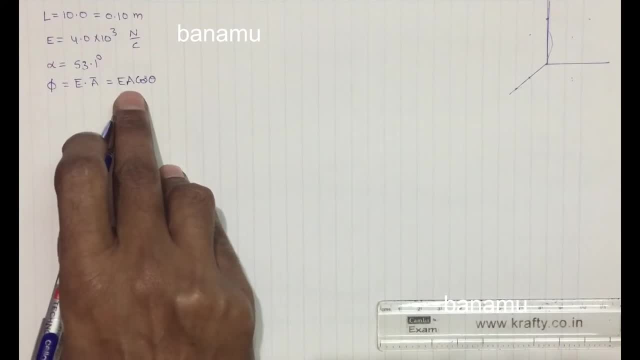 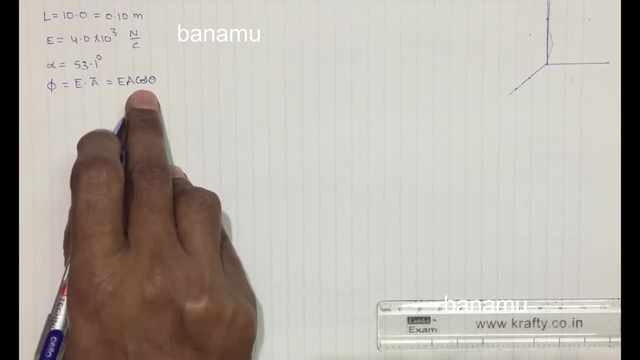 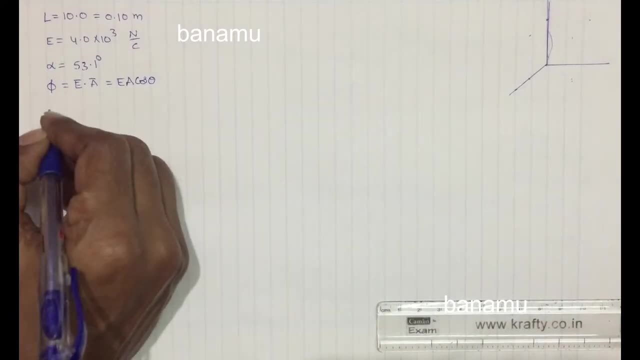 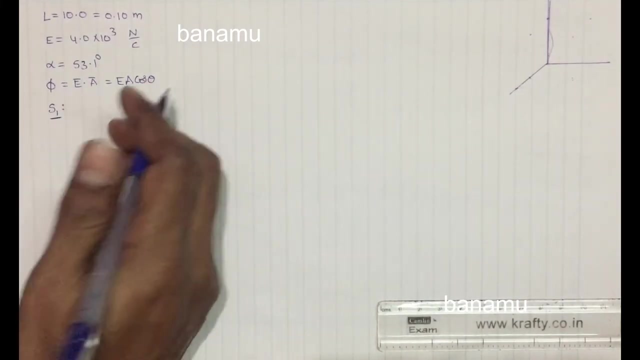 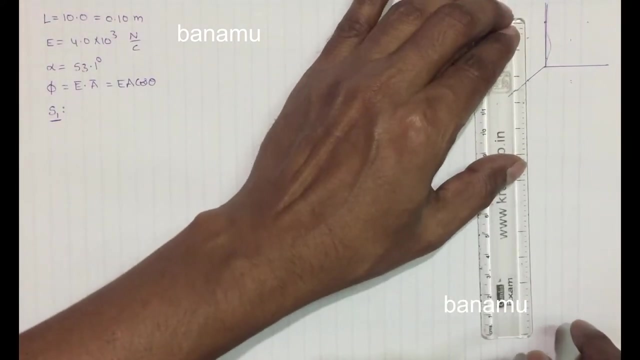 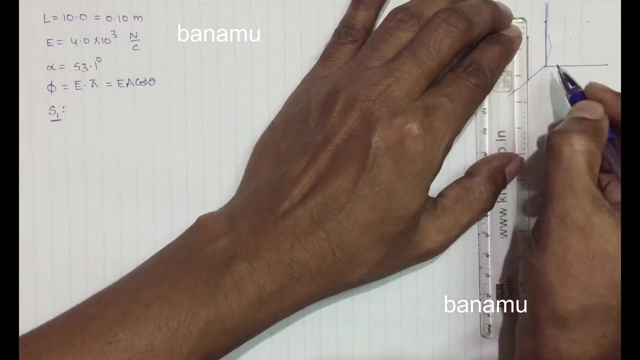 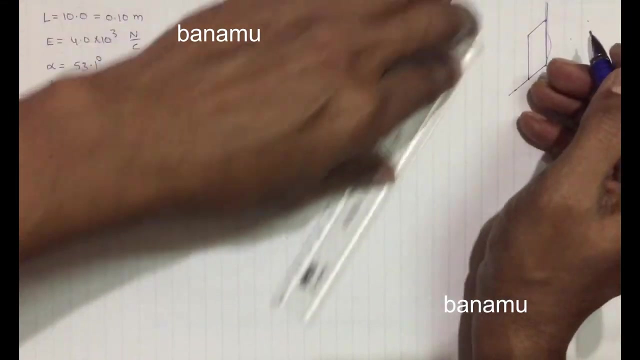 Where theta is the angle between the electric field and area. unit normal vector: the surface S1 in the figure. this is the left side of the cube. we can draw the figure surface S1. this is the surface S1. this is the surface S1 or. 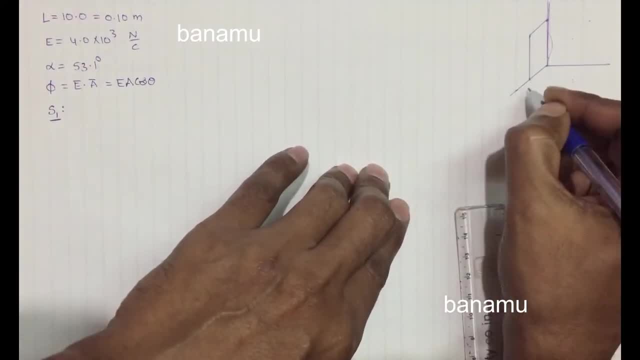 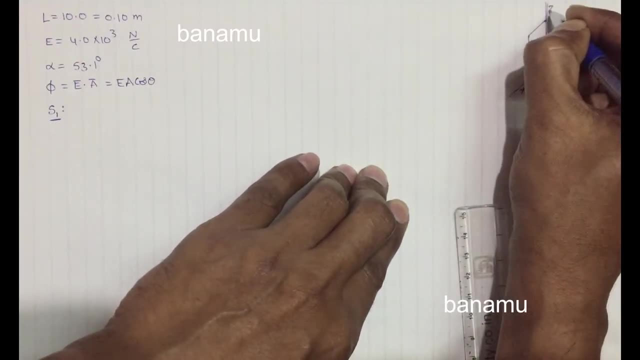 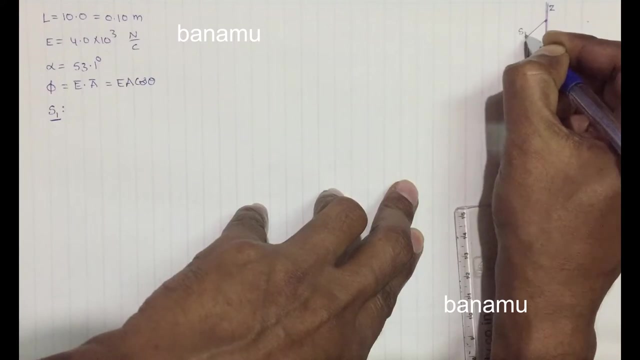 left side of the cube. let us take: this is the x-axis and this is the y-axis and this is the z-axis. so the surface S1. this is the surface S1. the surface S1 is the left side of the cube. first of all, the surface S1. this is the 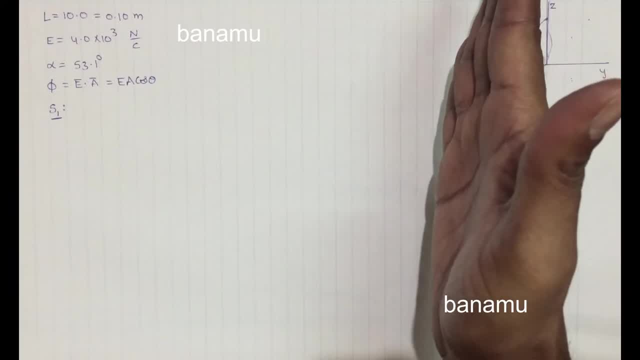 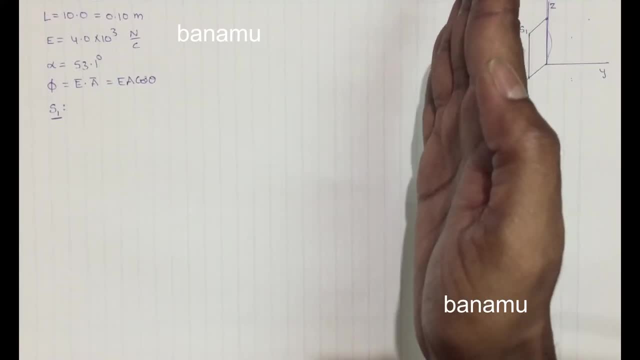 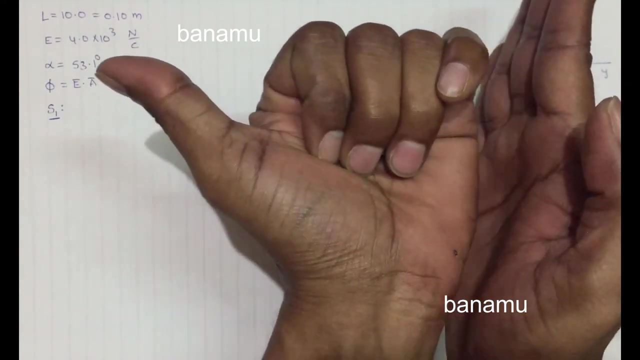 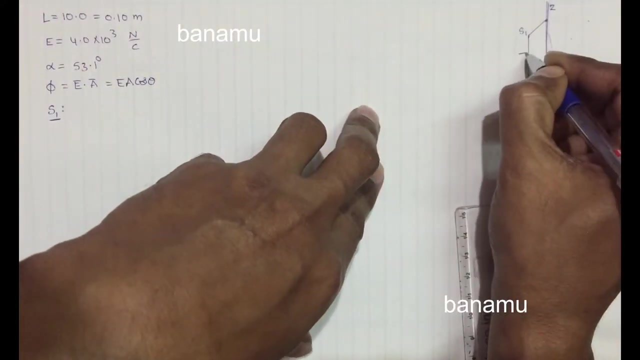 surface S1. the area unit normal vector along the perpendicular to the surface S1. so the area unit normal vector is perpendicular to the surface S1. so the thump direction is indicated. the area unit normal vector. okay, this is the. this is the area unit normal vector. 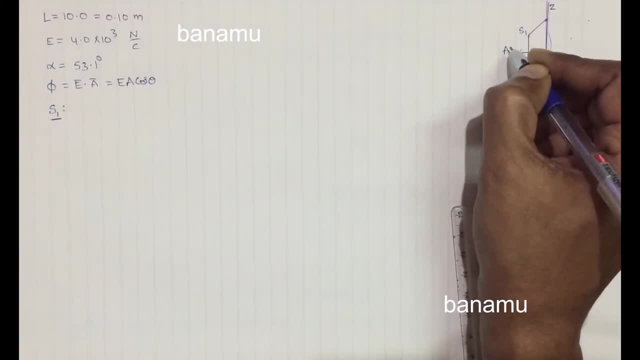 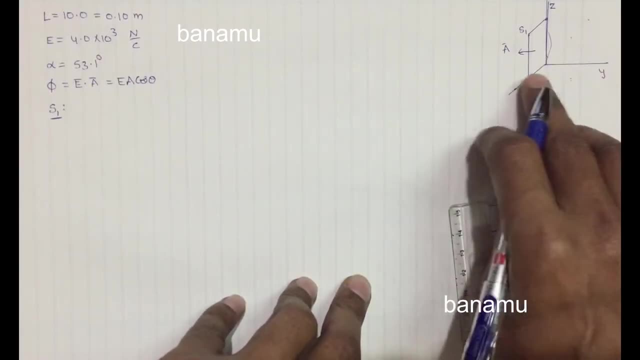 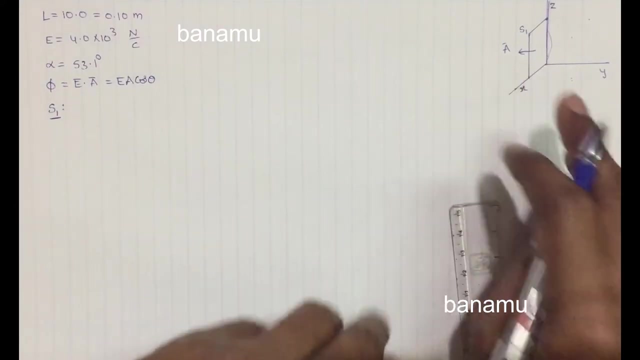 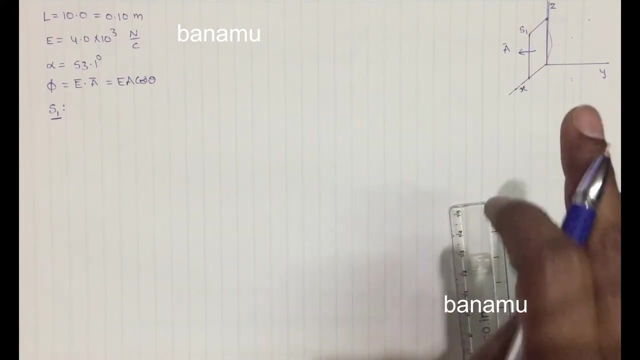 a bar or n cap. this is the area unit normal vector along the surface, along the parallel to the y-axis, negative y-axis. The area unit normal vector is parallel to the negative y-axis, So the angle between the- this is the angle between the electric field and area unit normal vector. 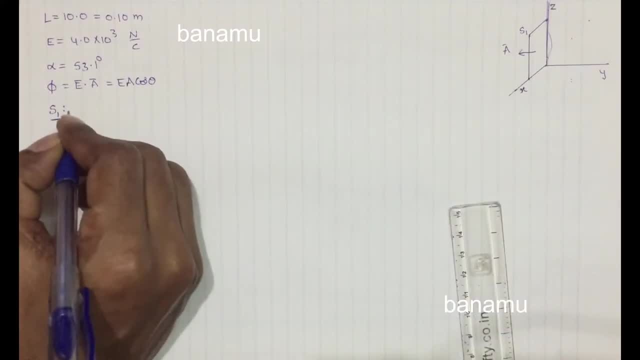 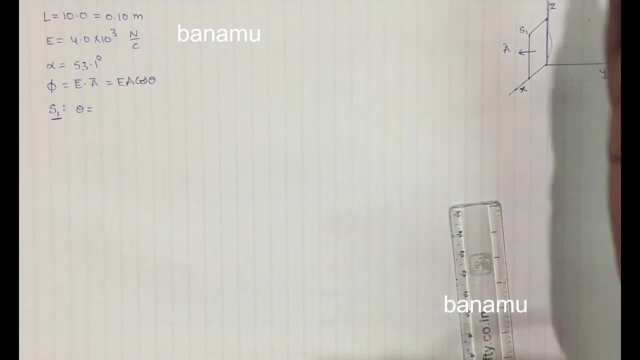 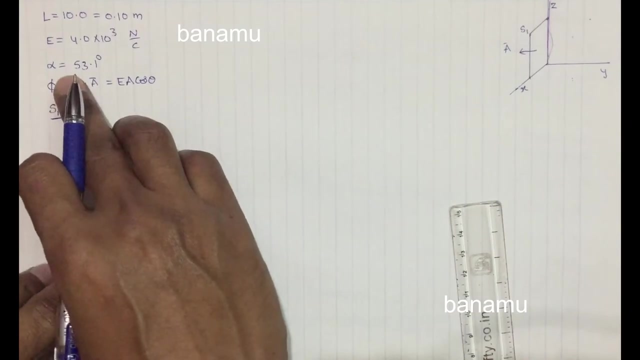 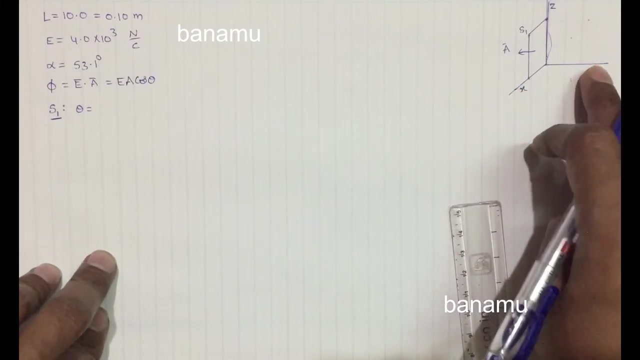 is the angle between the electric field and area unit normal vector. theta is equal to area unit normal. this is the area unit normal vector and the electric, where alpha is the angle between the electric field to xy plane, from x axis to y axis. So this is the direction. 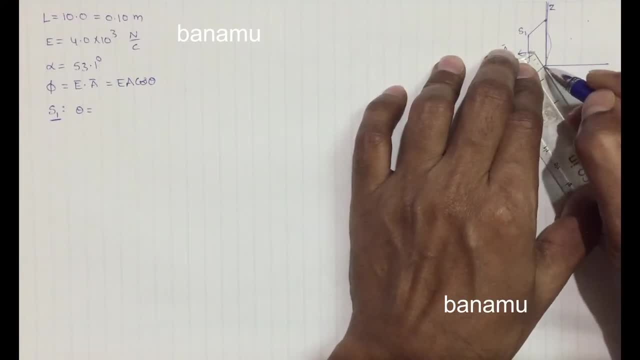 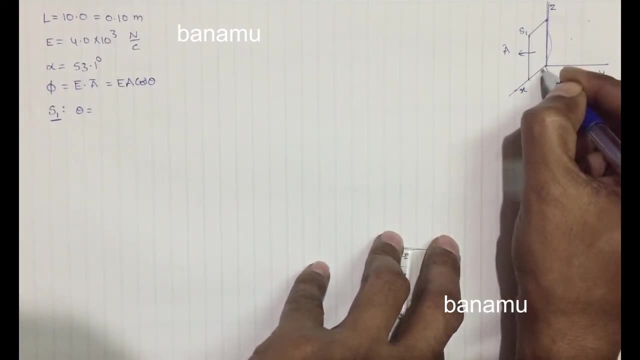 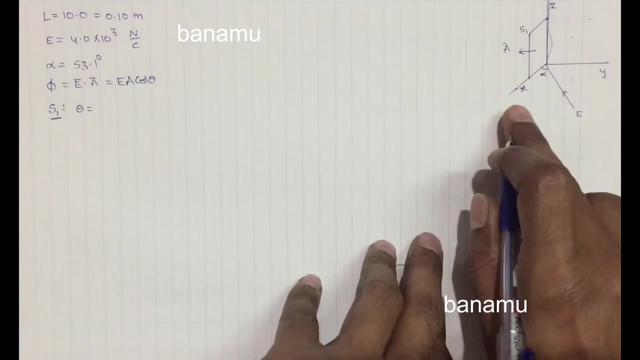 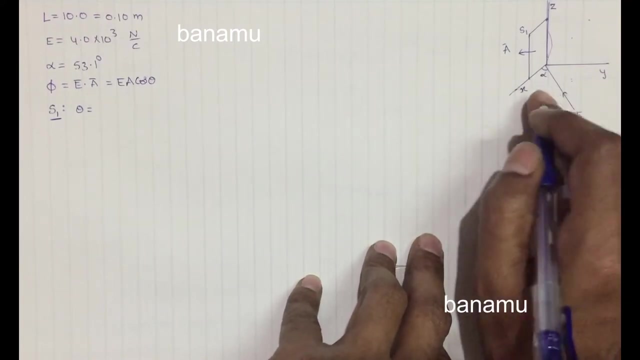 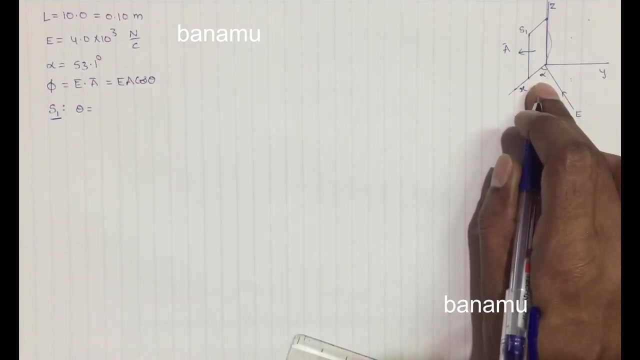 of the electric field. this is the direction of the electric field. the angle between this is the alpha. This is the electric field E, the angle between the x-y plane from the x-axis to y-axis, where alpha is the angle between the x-axis to electric field. E is alpha And we can draw. 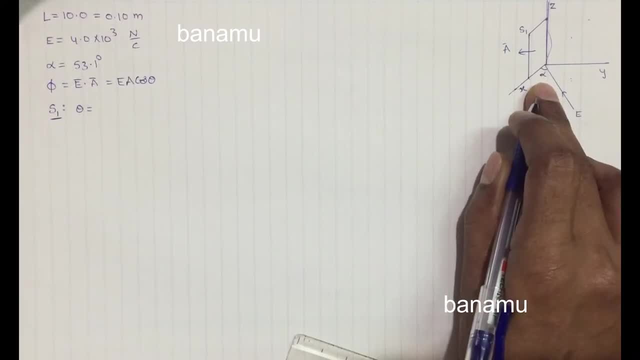 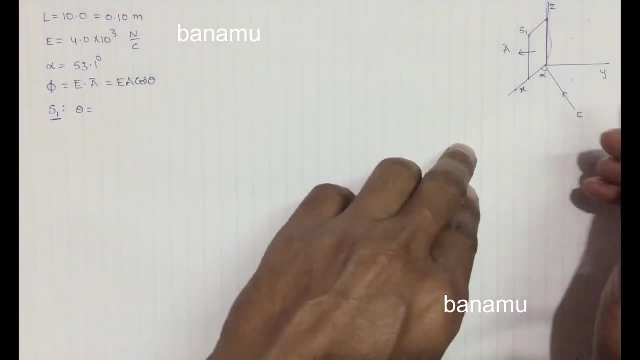 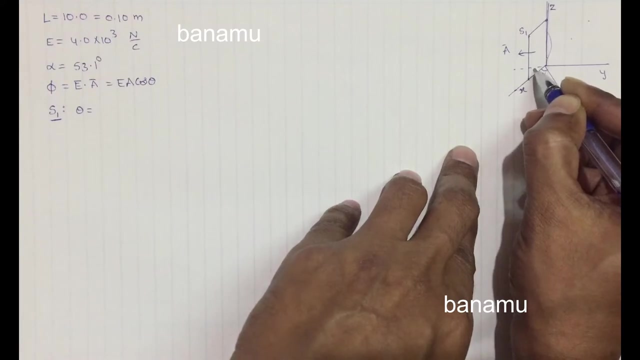 the electric field angle between the electric field and area unit normal vector is: this is the area unit normal vector. So the angle between the, the angle between the this line to the electric field is: this is the theta: The angle between the electric field to area. 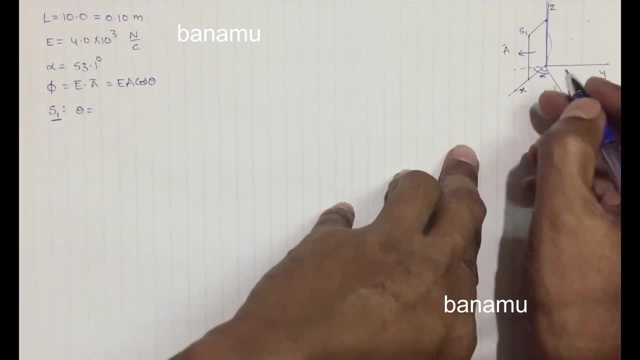 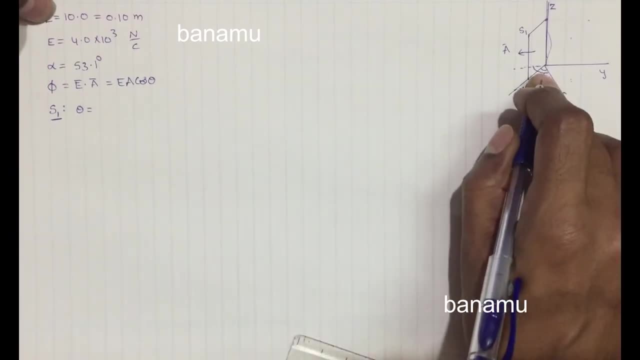 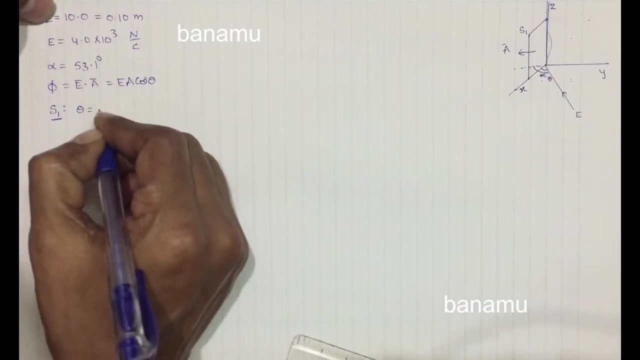 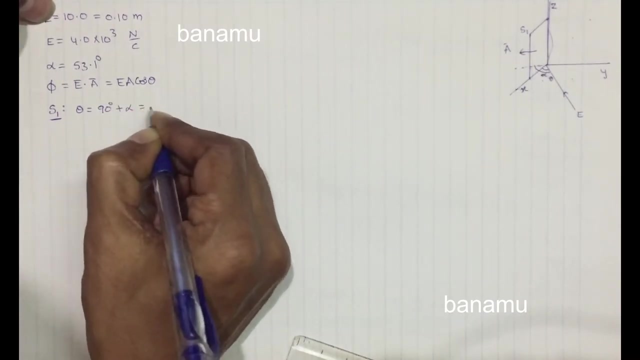 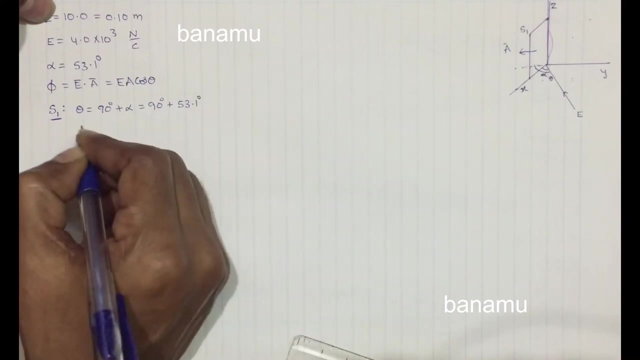 unit. normal vector to electric field is the theta. this is the theta. The value of the theta is theta is theta is equal to alpha, 90 minus alpha or 90 plus alpha, where theta is the 90 plus 90 degrees plus alpha, or 90 degrees plus 53.1 degrees. 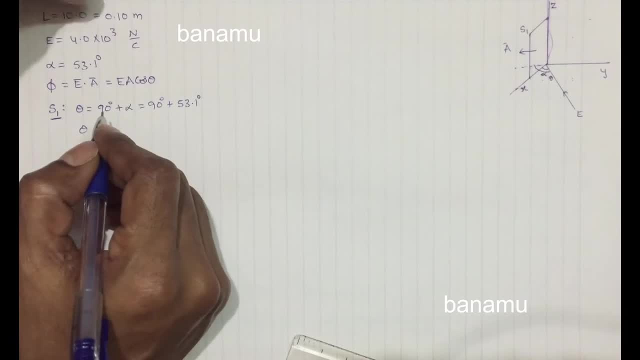 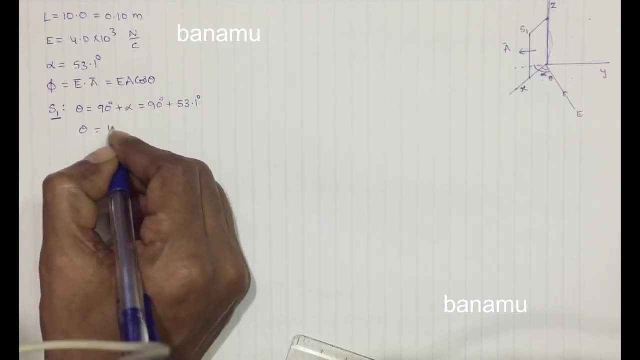 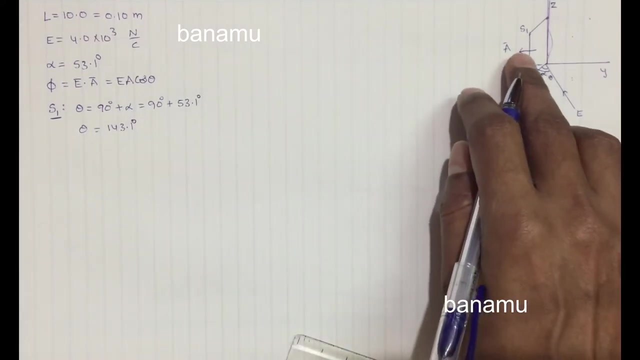 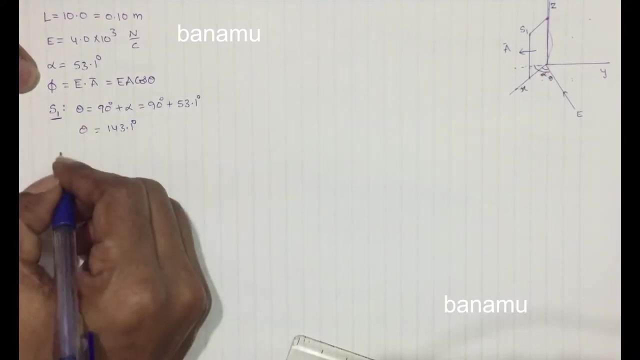 Theta is equal to 90 degrees plus 53.1 degrees is equal to 143.1 degrees. This is the angle between the area unit normal vector to electric field. So the electric flux at the surface S1 is the phi1.. Phi1 is equal to Ea. 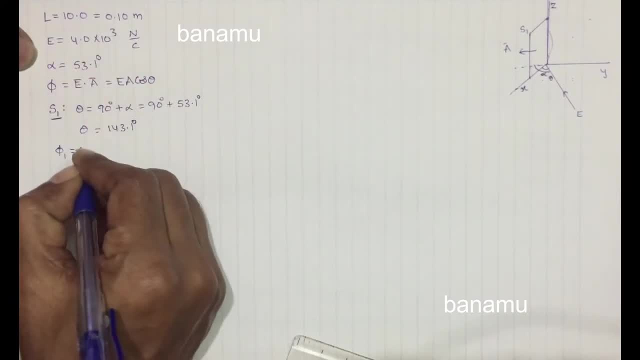 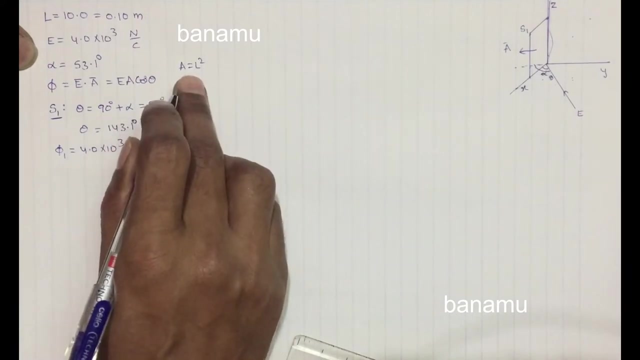 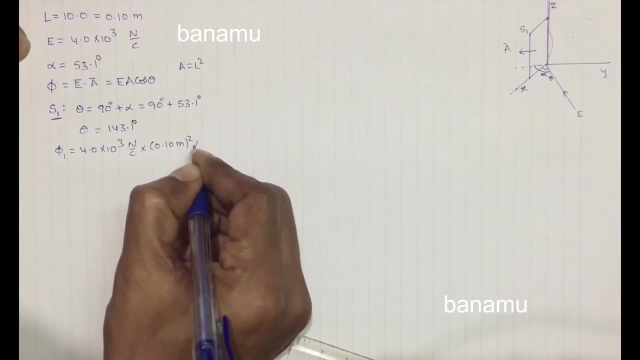 Ea, cos theta, where electric field is the 4 into 10 to the power of 3 Newton per Coulomb into area is the where area A is equal to L square. where area A is equal to L square, So 0.10 meter whole square into cos theta is the 140.1 degrees. 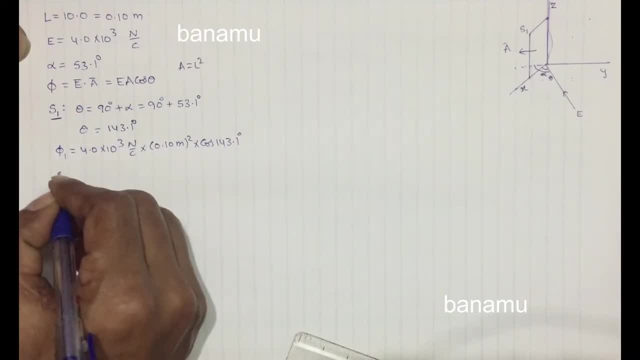 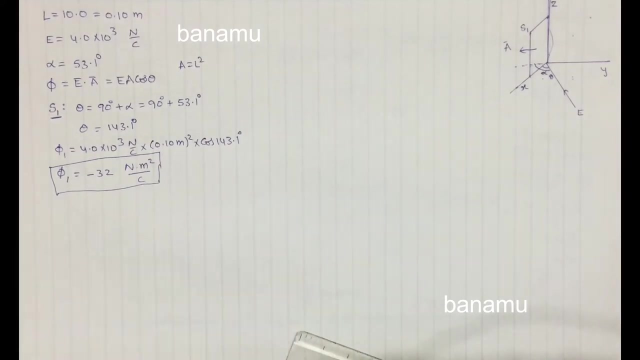 So phi1 is equal to. phi1 is equal to minus 32 Newton meter square per Coulomb. This is the electric field at the surface S1.. This is the electric flux at the surface S1.. And consider the electric flux at the surface. 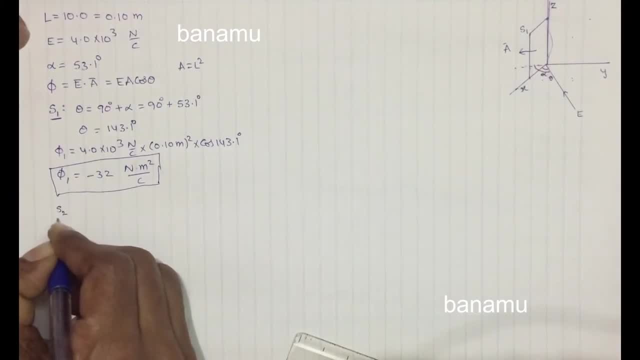 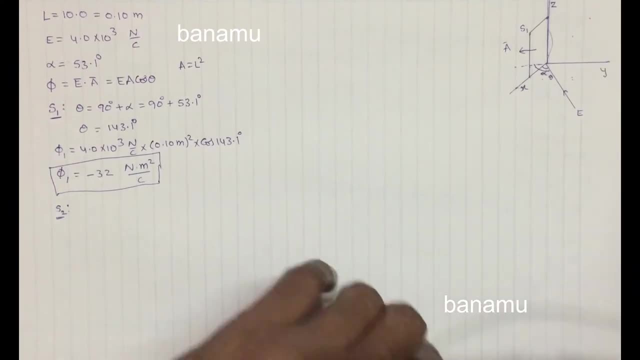 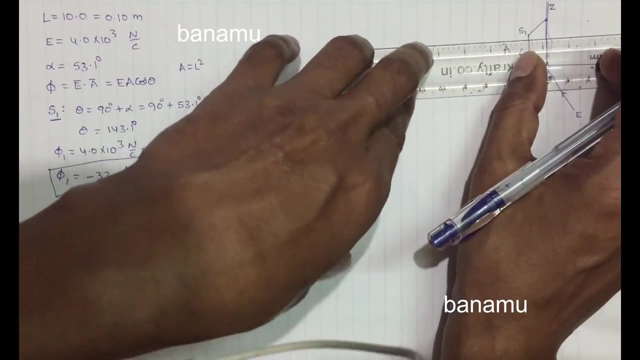 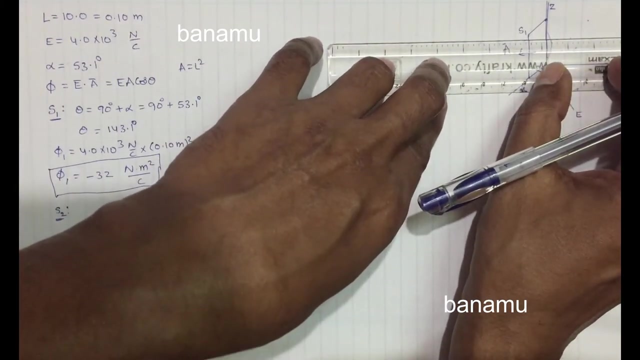 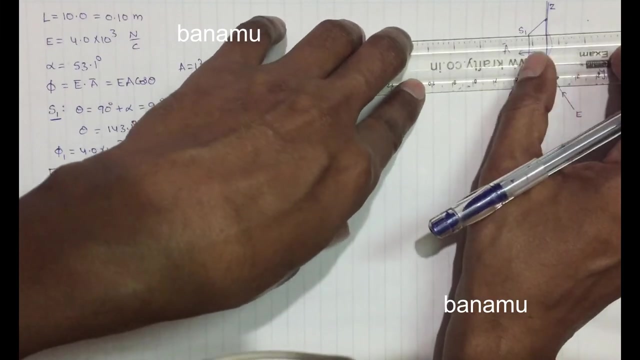 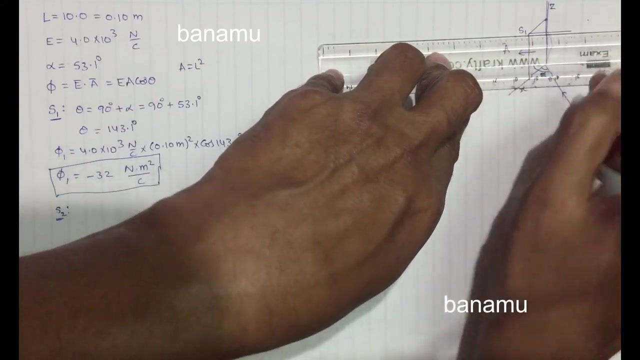 Another one is the electric flux at the surface S2.. The surface S2 is the from the figure. this is the surface S2 is the upper part of the cube. upper part of the cube. This is the upper part of the cube. 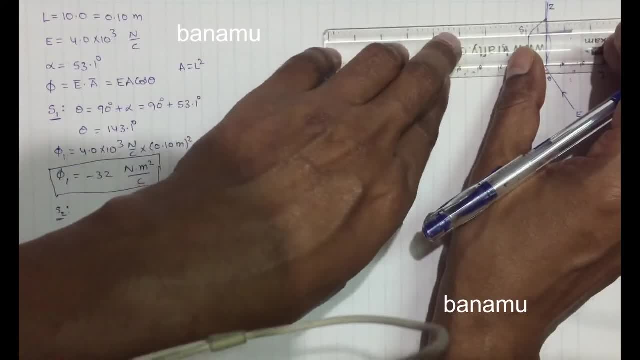 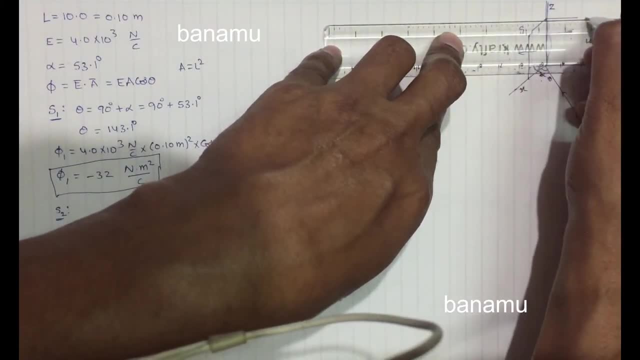 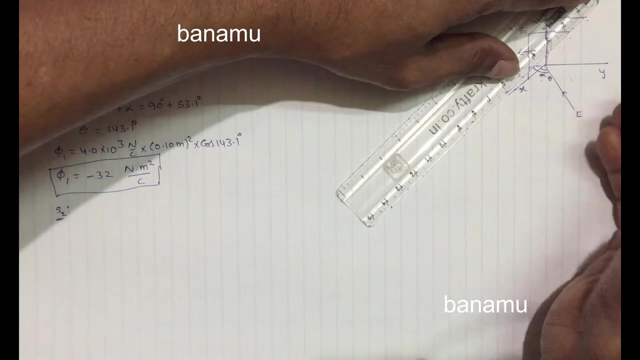 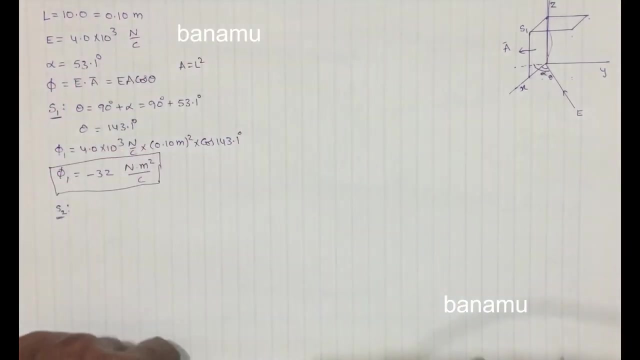 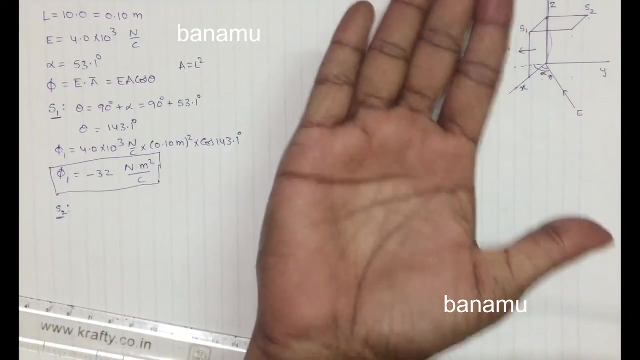 This is the surface H2.. This is the surface S2.. The surface S2.. S2 is the upper part of the cube. This is the surface S2.. The surface S2 is the upper part of the cube. This is the surface S2.. This is the surface S2.. The surface S2, the unit normal. 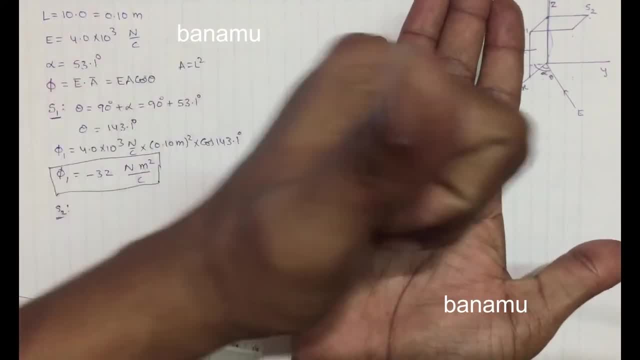 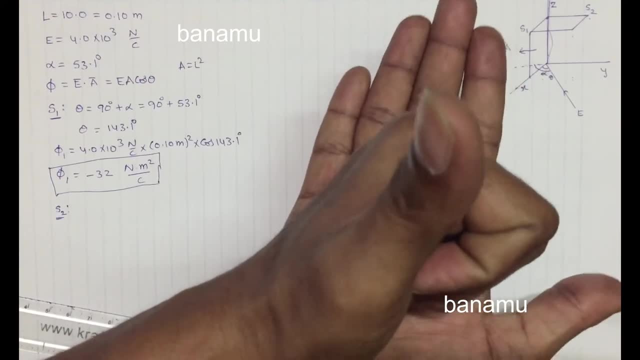 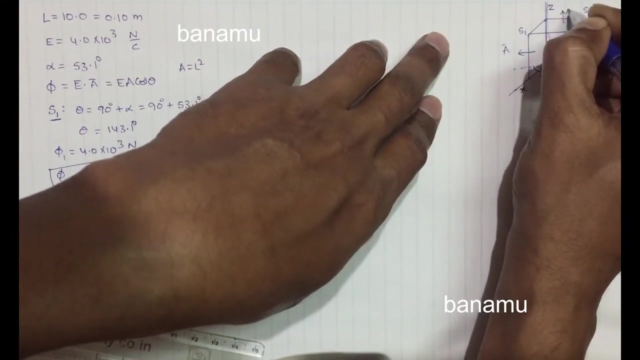 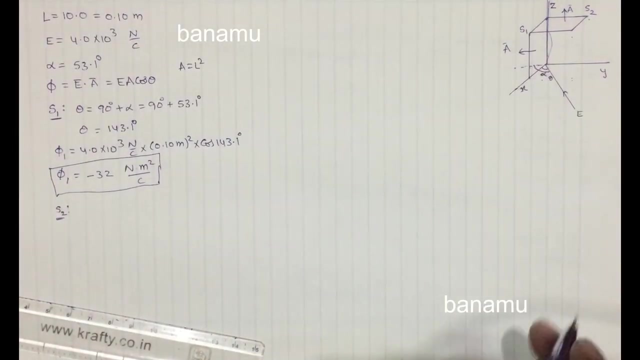 vector of the surface. S2 is perpendicular to the surface. So this is the thumb direction, indicates the area unit. normal vector of the surface. So the direction of the area unit. normal vector A bar is this direction upward of the cube. So the angle between the area. 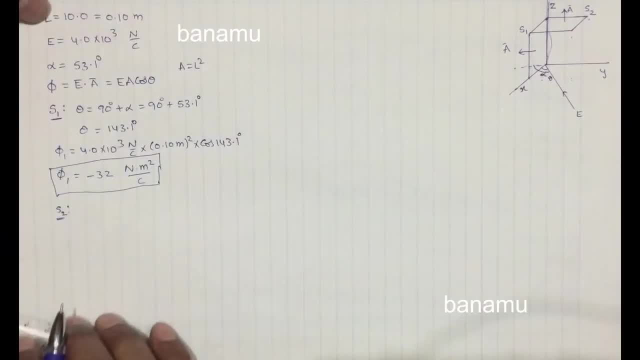 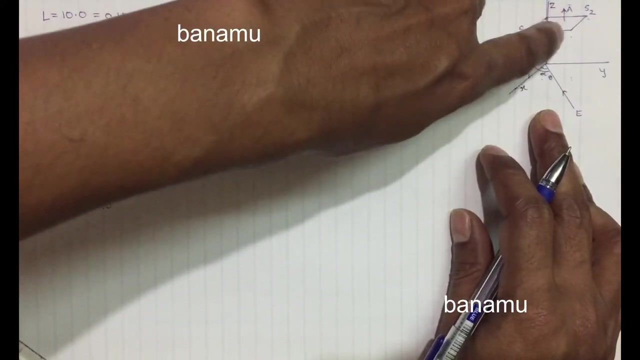 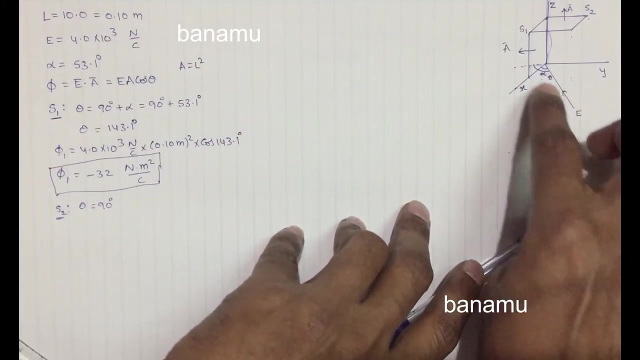 unit normal vector to electric field is 90 degrees, So alpha theta is equal to 90 degrees. This is the area unit normal vector is parallel to the positive z axis, So the electric field is the electric field along the xy plane. So the angle between the xy plane to z axis. 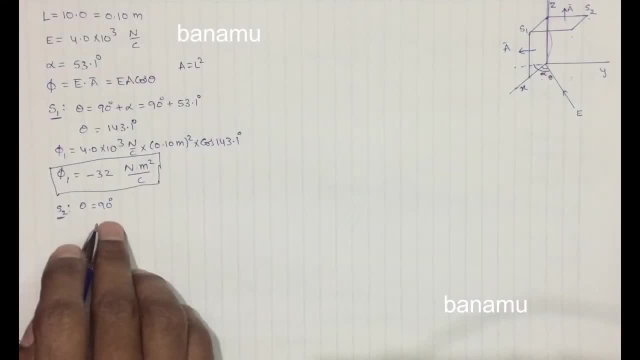 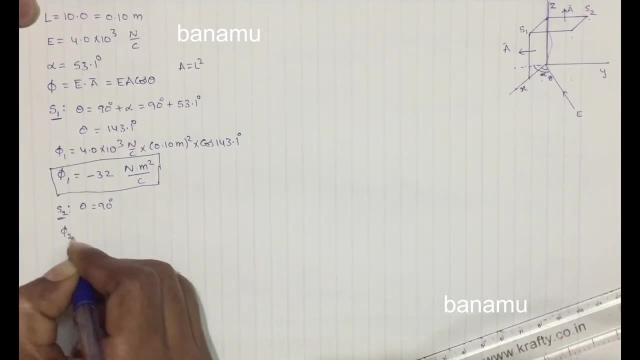 is the 90 degrees, So theta is equal to 90 degrees. Finally, the electric flux, phi 2 is equal to E, A, cos, 90 degrees, 4 into 10, to the power of 3 newton per coulomb into 0.1 meter, whole square into. 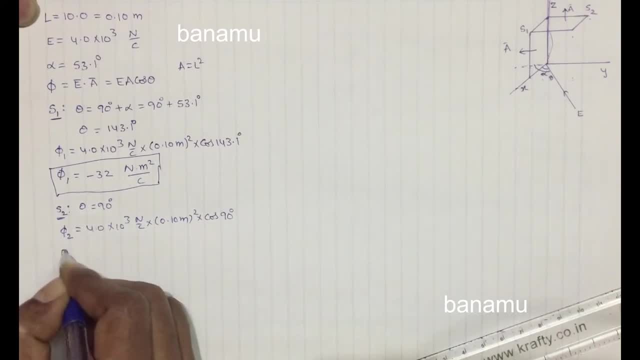 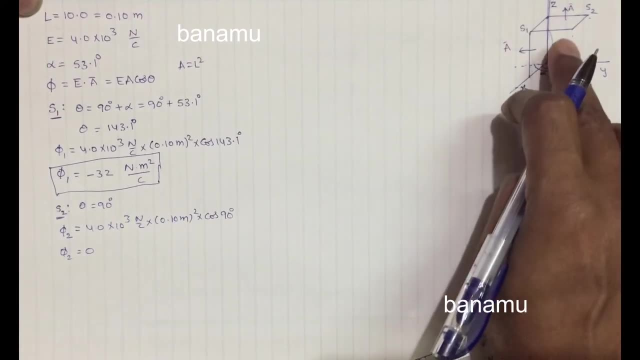 cos 90 degrees. Phi 2 is equal to 90 degrees. Phi 2 is equal to 0 because the angle between the electric field to area unit normal vector is perpendicular to each other. So cos 90 is equal to 0.. 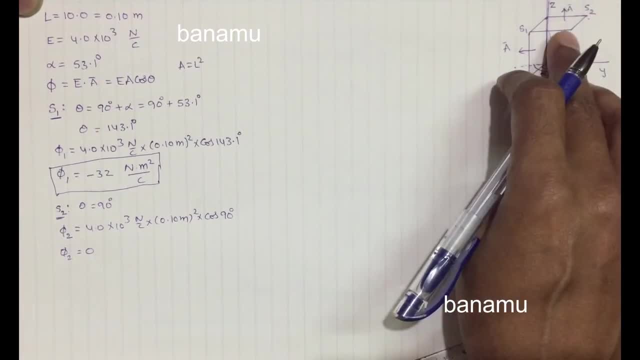 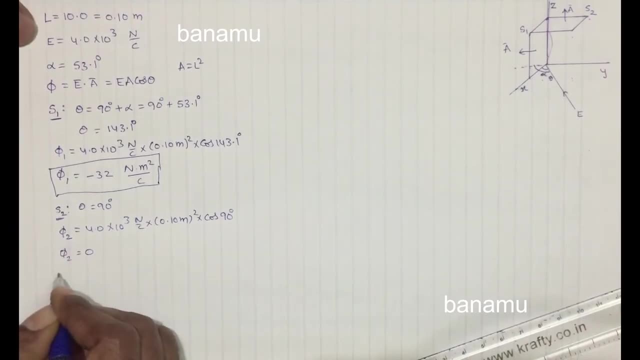 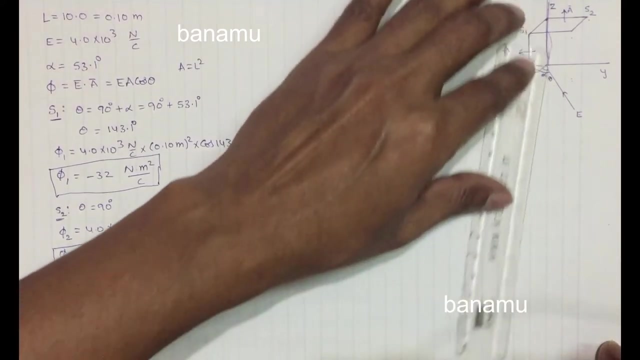 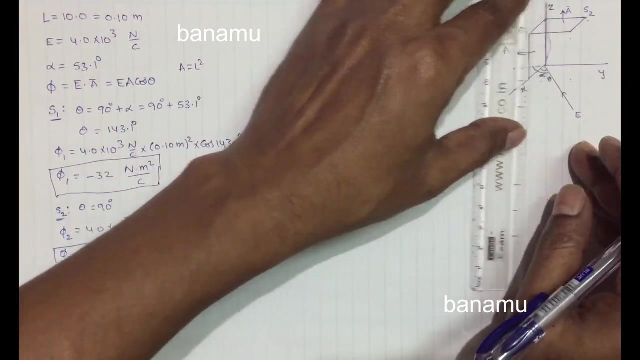 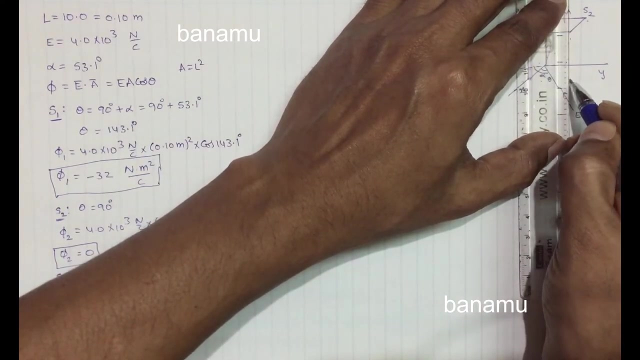 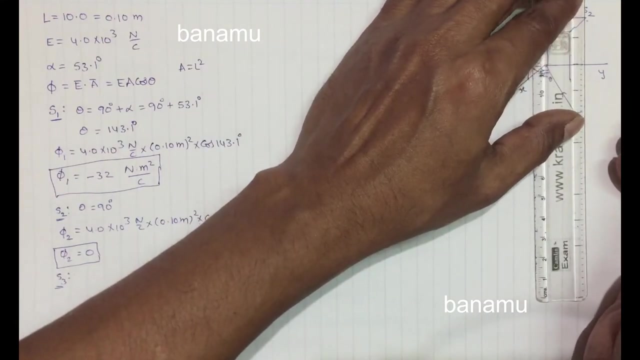 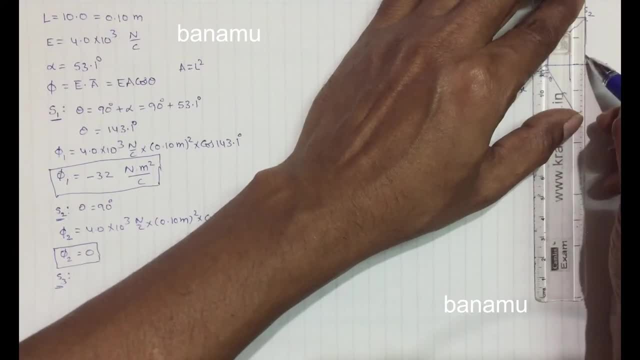 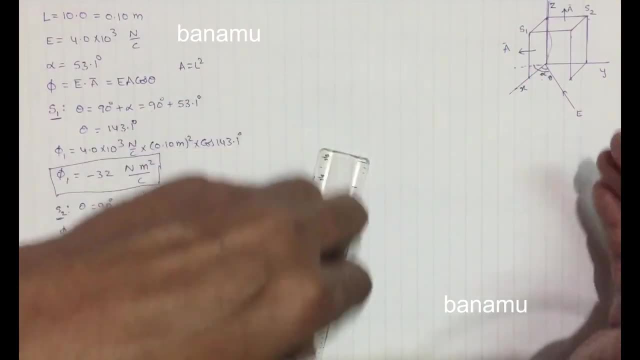 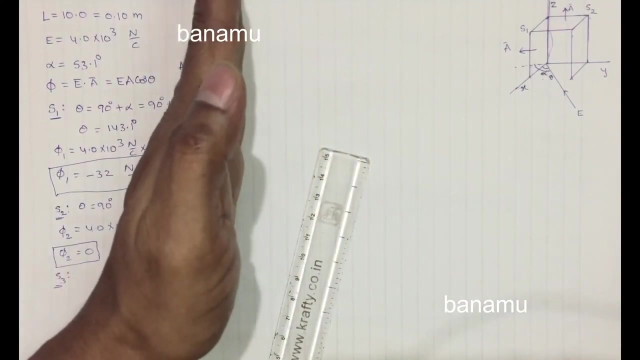 is the right side of the cube, So this is the surface S3.. This is the surface S3.. The surface S3 is the right side of the cube, So this is the surface S3.. So in this case, 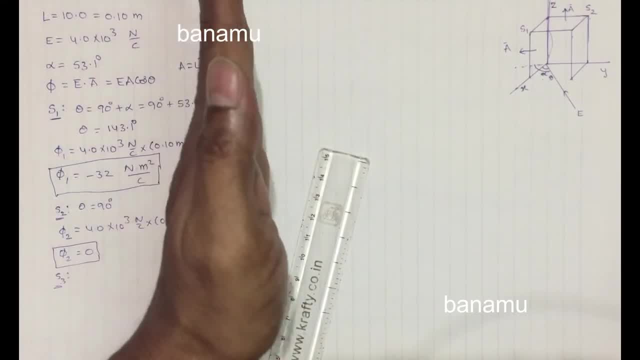 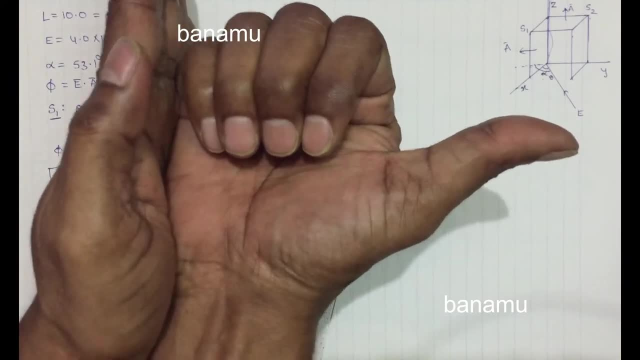 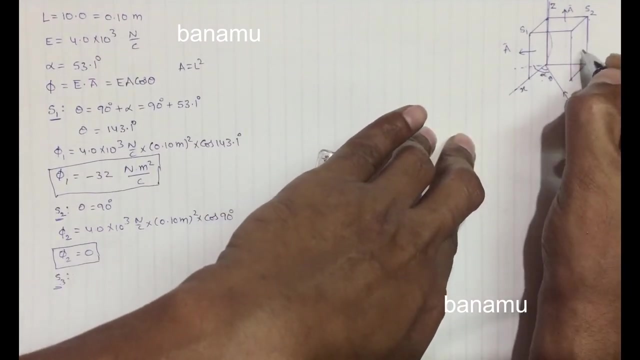 the area unit normal vector is perpendicular to the surface, So the surface is perpendicular to the. the thumb direction is indicated the area unit normal vector, So the direction of the thumb along the positive y-axis. So the surface of the, the area unit normal vector. 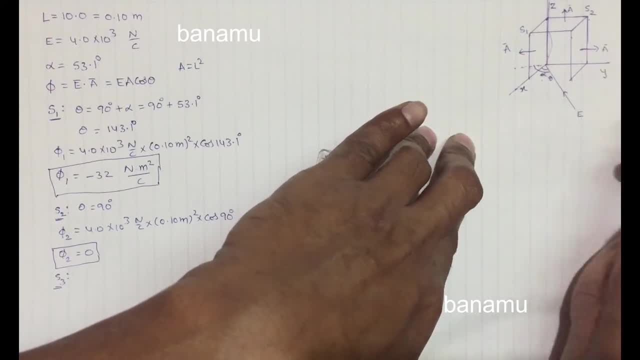 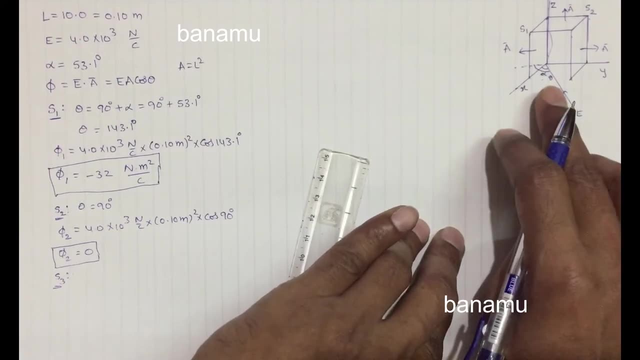 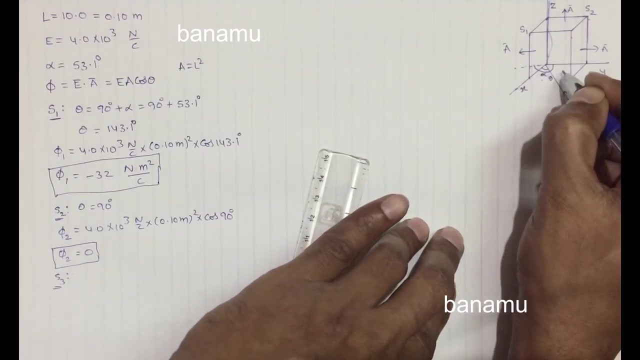 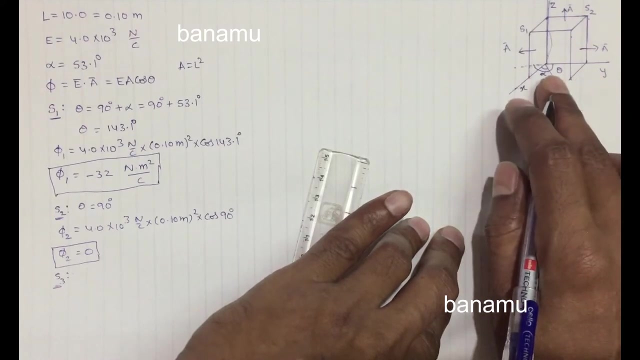 is along the positive y-axis, So the direction along the y-axis, So the angle between the the electric field to y-axis is the. this is the. this is the theta. This is the theta. The angle between the electric field to area unit normal vector is the theta. 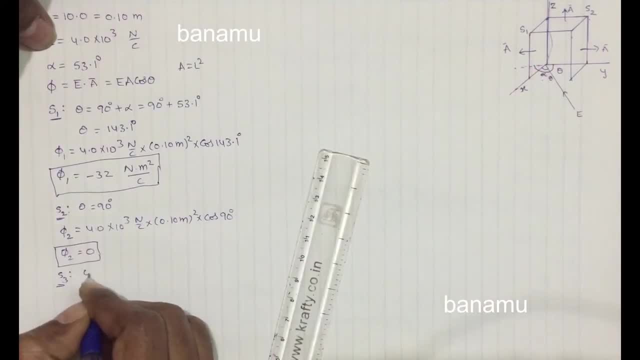 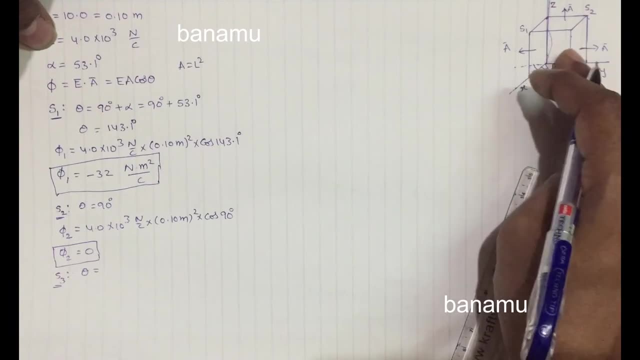 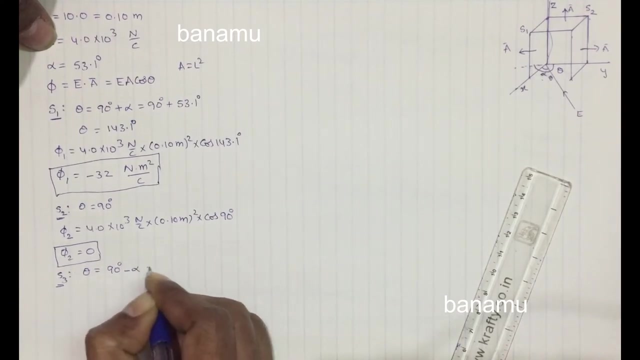 Theta is. the theta is equal to. this is the: the angle between the electric field to area unit: normal vector. That is equal to 90 degrees minus alpha. That is equal to 90 degrees minus alpha is the 53.1 degrees. 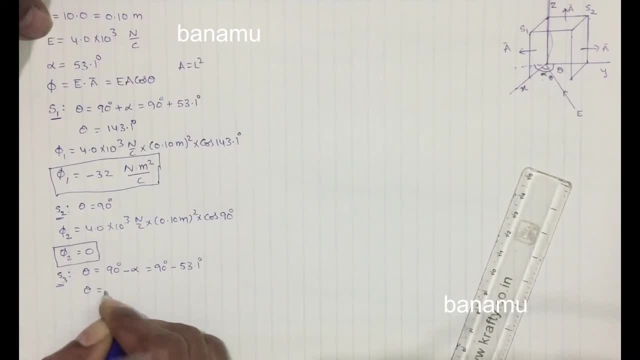 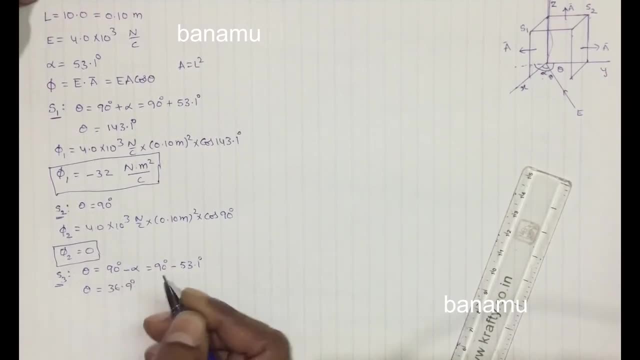 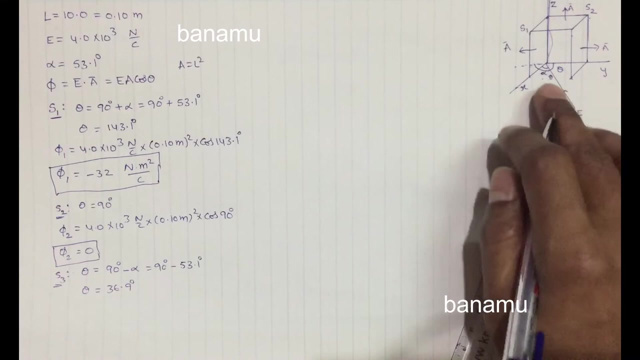 So theta is equal to 36 point where theta is equal to 36.9 degrees. This is the theta because the electric field along the xy plane, So angle between the x-axis to electric field is the alpha And we can calculate the angle between the y-axis to electric field is the 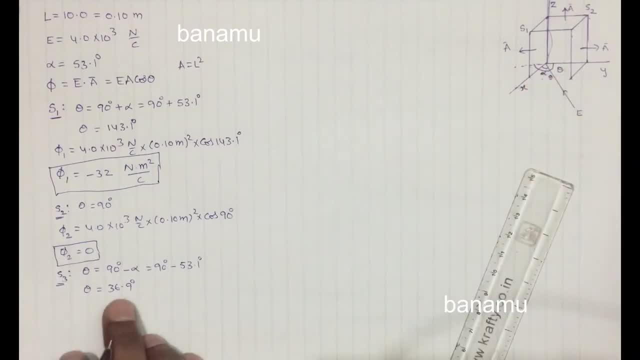 90 minus alpha, So it gives to the theta. So theta is equal to 90 minus alpha, or 90 minus 53.1 degrees is equal to 36.9 degrees. So the electric flux at the surface S3 is the phi 3.. Phi 3 is equal to E A cos theta. 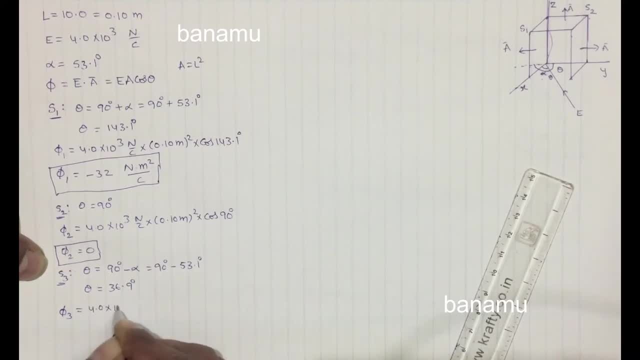 The electric field E is equal to 4 into 10, to the power of 3 Newton per coulomb into area is the L square, the electric field E is equal to 3 N square, So delta S3 is equal to 3 S2 per douA. 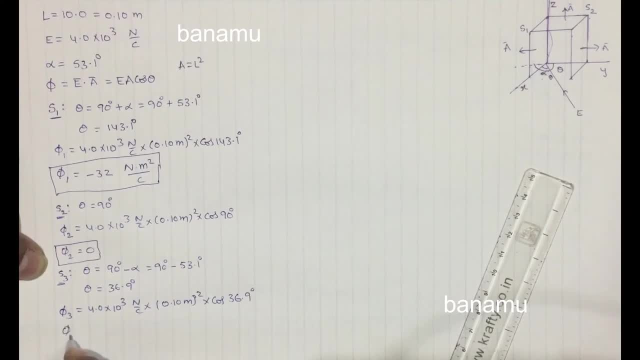 the electric flux at the surface S3 is equal to 8 E A cos theta. This is the electric flux at the surface, So delta E is equal to 4.. So this is the power of E- B when we calculate this area. 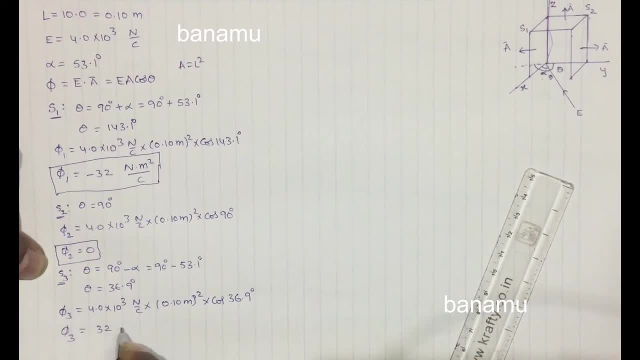 And now income fromищa is x ou volume divided by E cMar練. So delta plus hyper chi by dou T c comma Gx is equal to this is, which is encontrar ultra and T mi squared pi. 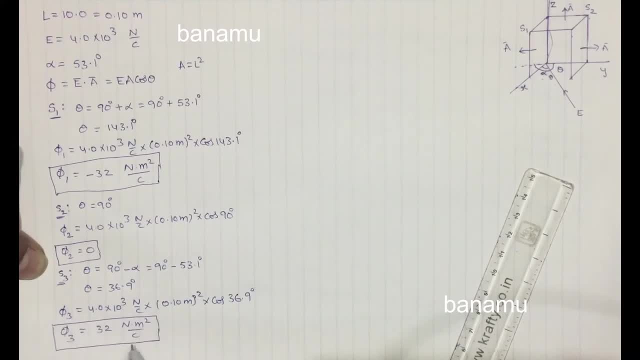 which isoh überhaupt. before redeem or extra, the home constant is equal to redarlo. this is the. this is metaphysical effect. in baraje update is equal to u bi over ensemble S3.. This is the electric flux at the surface, S3.. And another one calculate the electric. 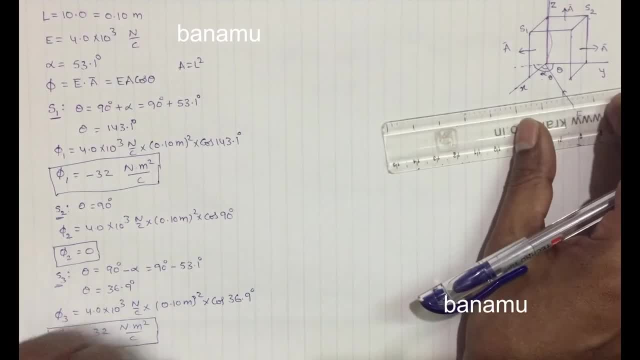 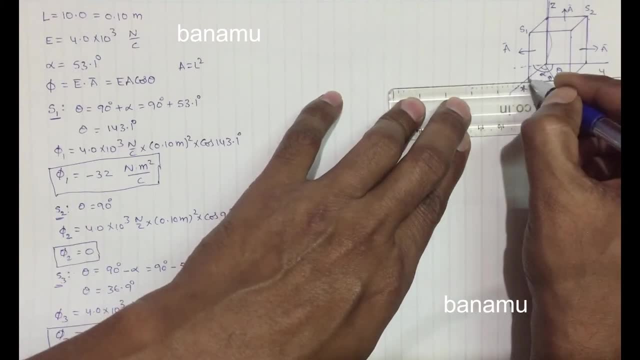 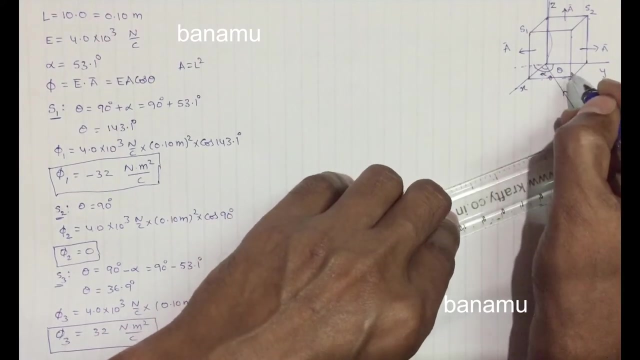 flux at the surface S4.. Draw the figure: the surface S4.. Draw the figure: the surface S4.. This is the surface S4.. This is the surface S4.. This is the surface S4.. So this is the 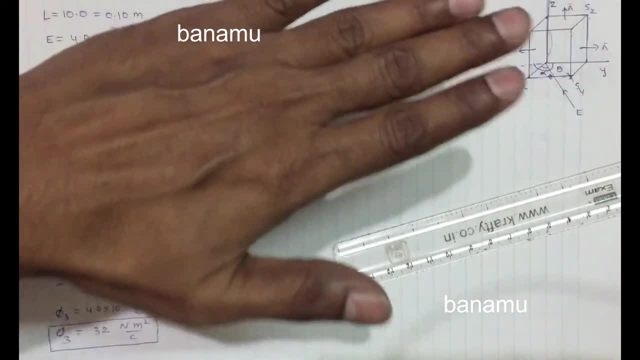 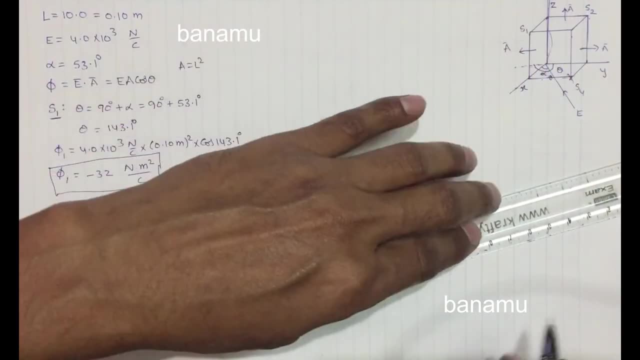 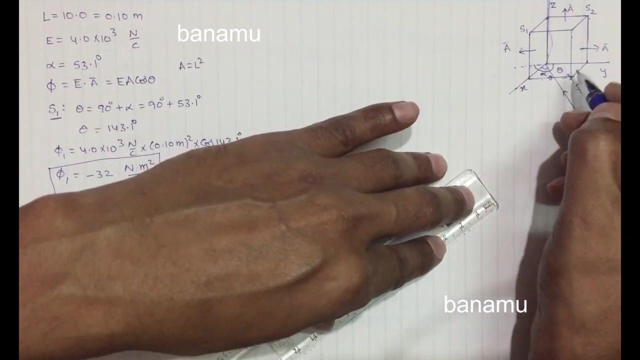 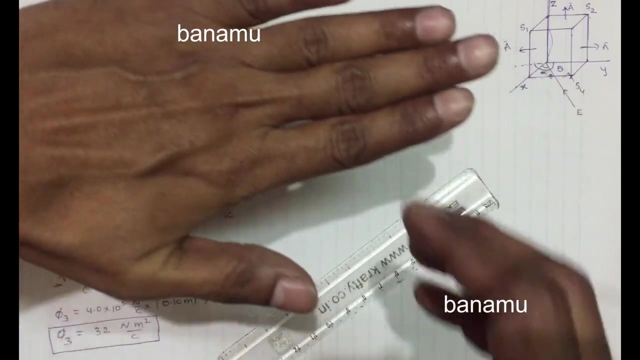 surface S4.. The surface S4 are the downward of the cube, Downward of the cube. This is the surface S4.. So the unit normal vector, rather the unit normal vector, the unit normal vector is the downward of the cube. So the unit normal vector is perpendicular to the surface. So the unit 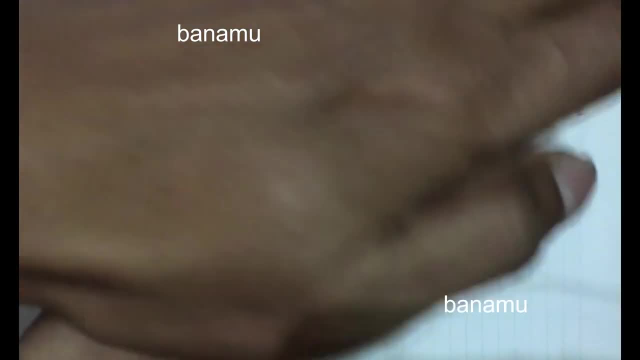 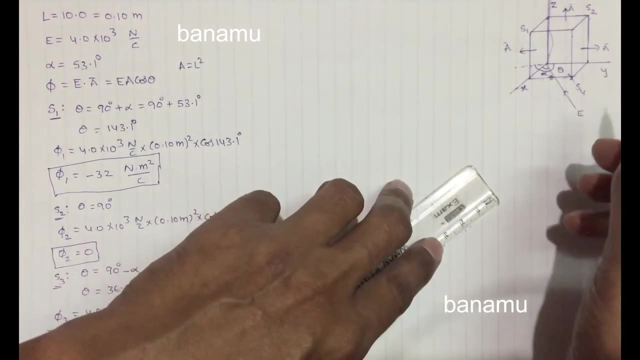 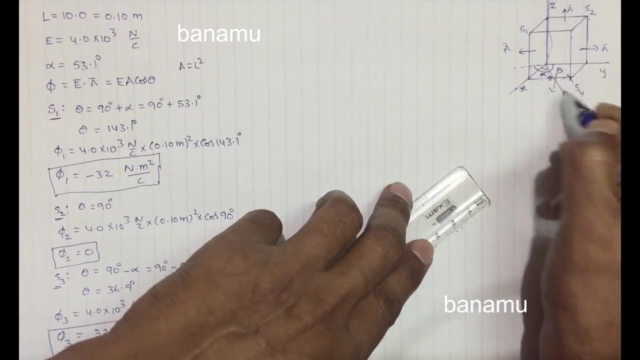 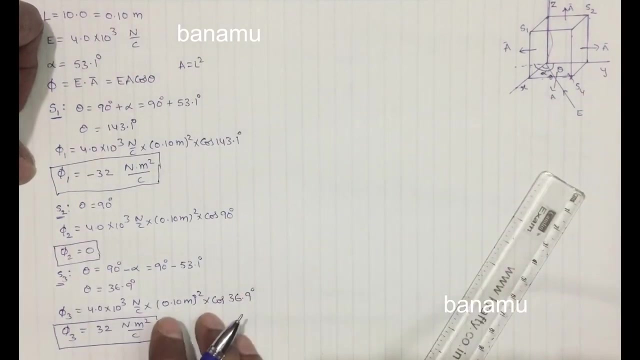 normal vector is indicated: the direction of the thumb. So this is the direction of the thumb downwards to the cube, or negative z axis. So the electric field toward the negative z axis. This is the. So the angle between the electric field to area unit normal vector is: 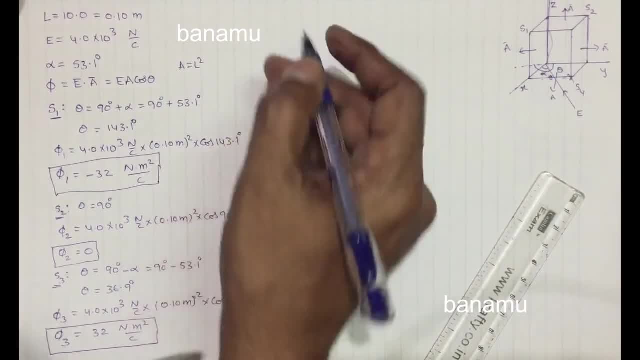 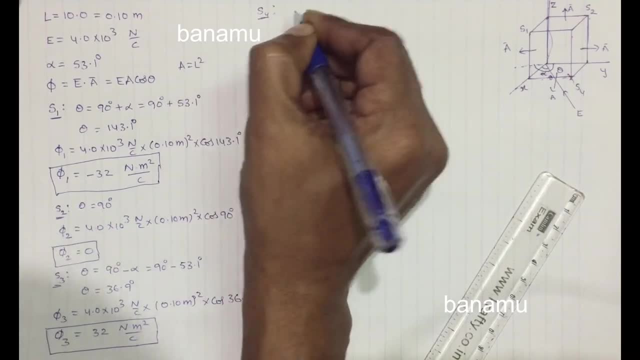 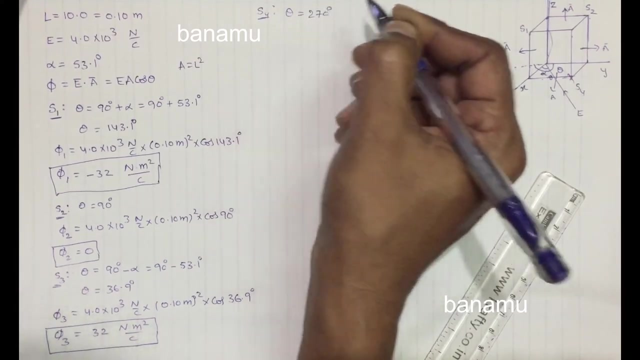 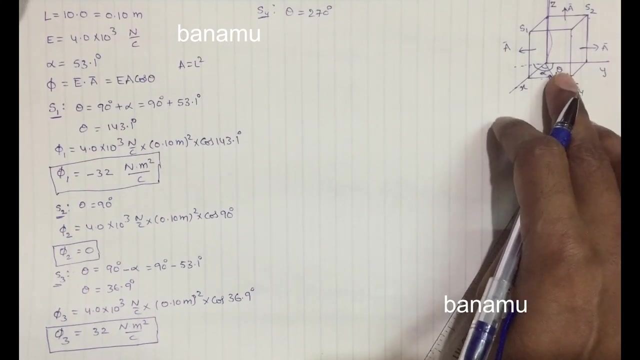 90 degrees or 270 degrees. So consider the surface S4 where theta is equal to. theta is equal to 270 degrees. The angle between the electric field and the area unit normal vector is 90 degrees. field to area in unit normal vector at the surface S4.. The surface S4 is the. this is: 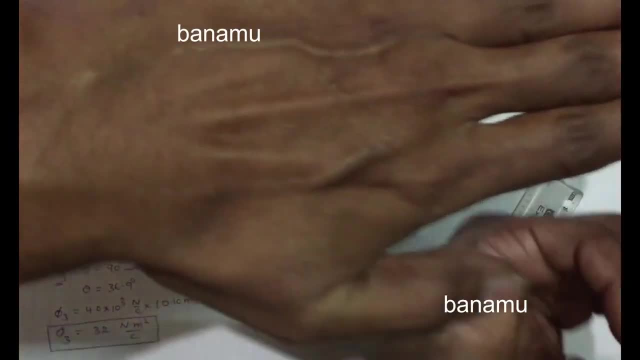 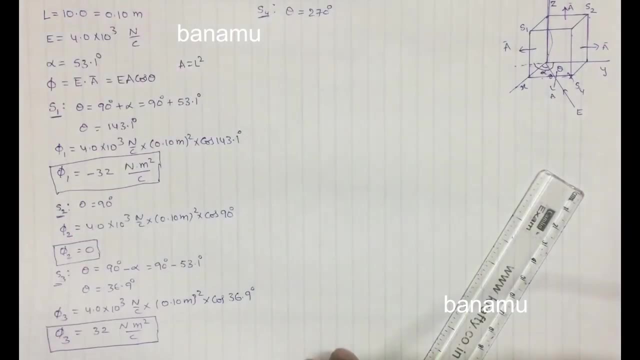 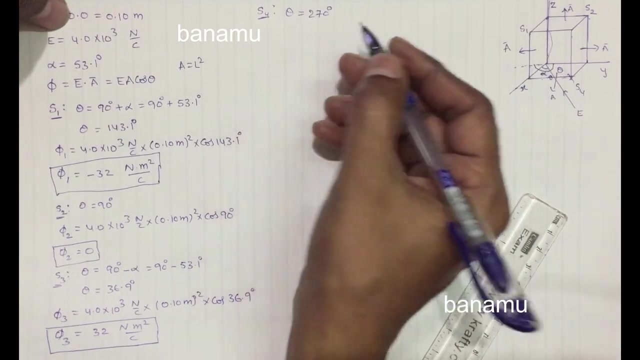 the surface S4. So the unit normal vector is downwards to the surface S4. So the thump direction is indicated towards the unit normal vector. So angle between the electric field to unit normal vector is: theta is equal to 270 degrees. So the electric field, the electric 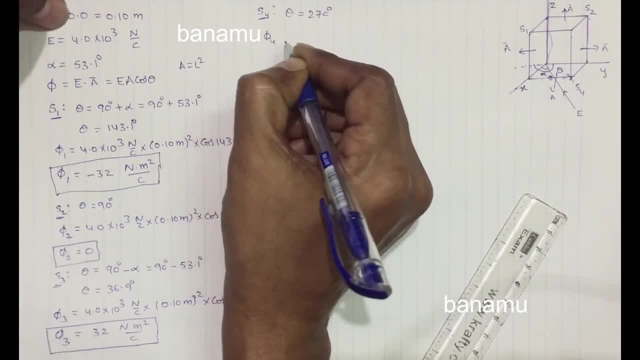 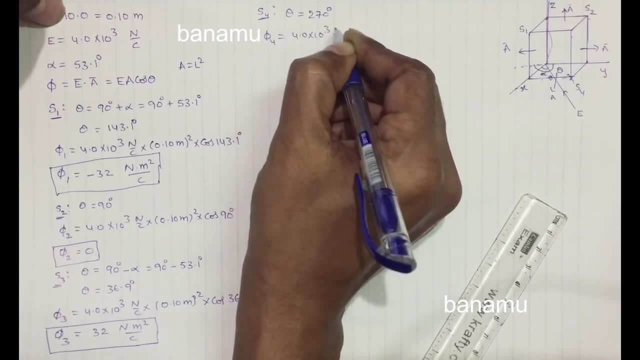 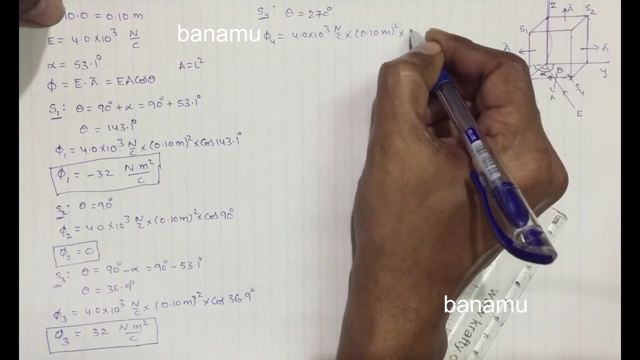 flux at the surface 5, 4 is equal to E. value of the E is equal to 4 into 10 to the power of 3 Newton per coulomb. into area is the 0.1 meter whole square into cos. theta is 270 degrees. 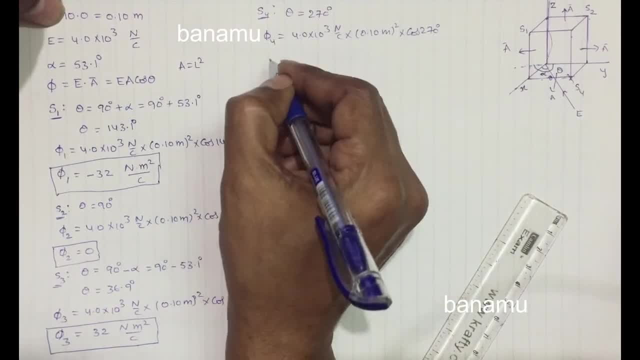 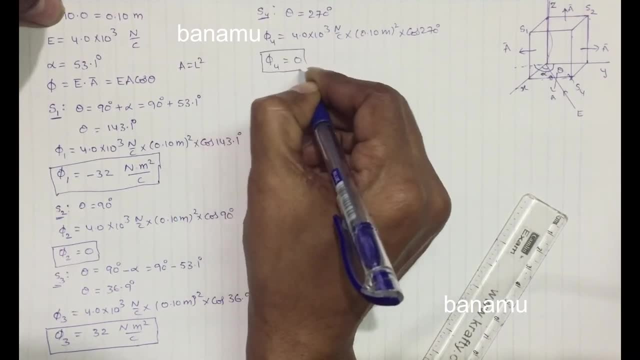 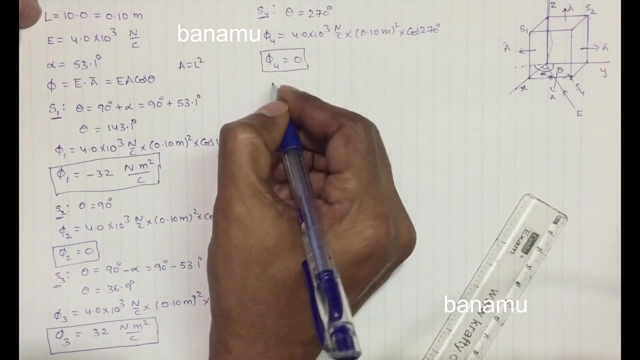 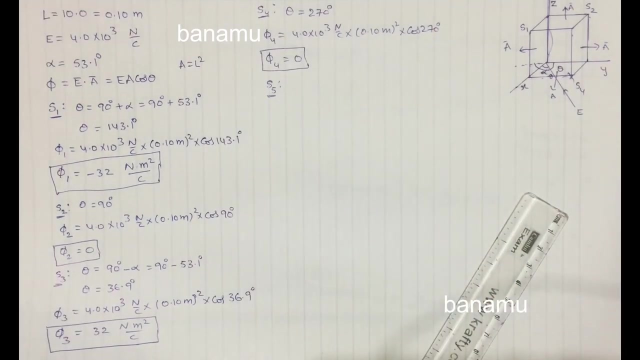 So cos 270 is equal to 0.. So the electric flux at the surface S4 is equal to 0.. This is the surface S4 and we can calculate the surface S5.. This is the surface. we can calculate the surface S5, where surface S5 is the front of the cube. This is the surface. 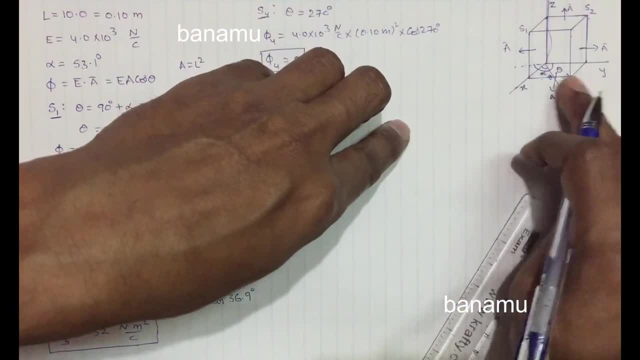 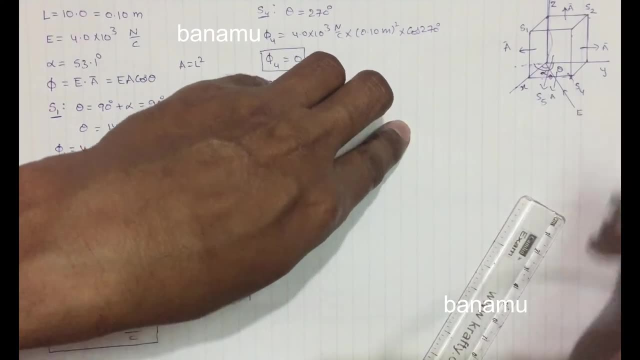 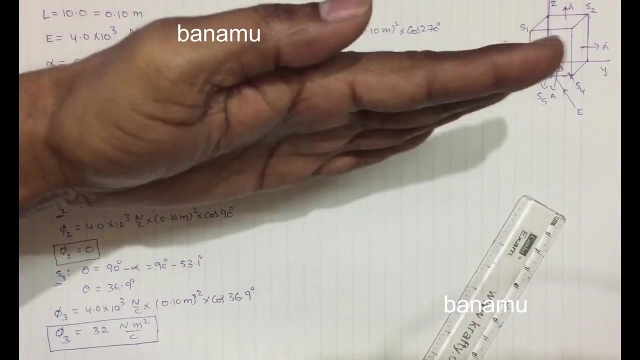 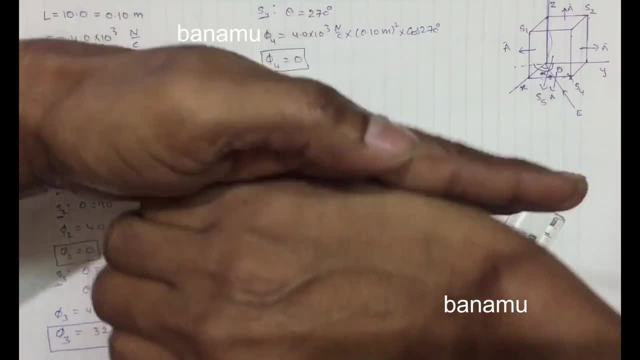 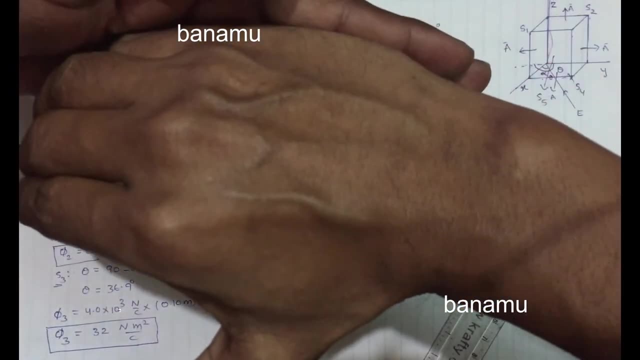 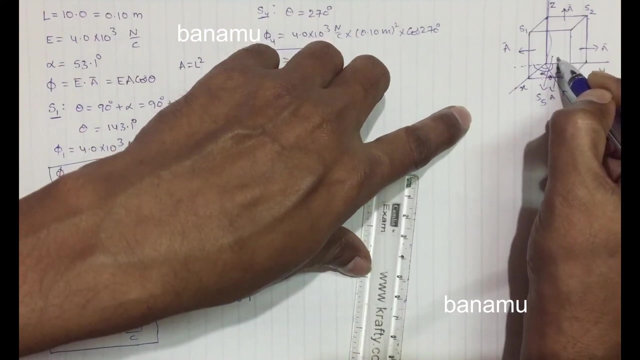 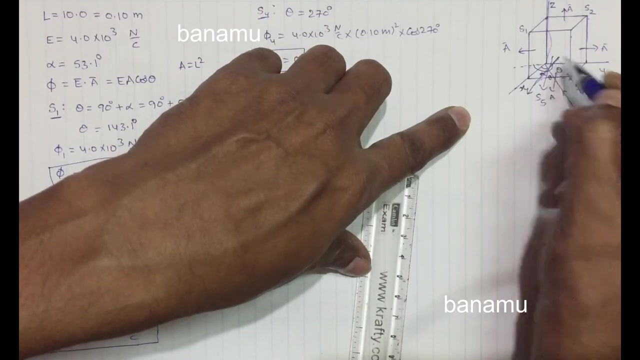 the x-axis. so this is the unit normal vector- is perpendicular to the x-axis. so this is the thumb indicates the unit normal vector direction. so the angle between the unit normal vector. this is the unit normal vector, this is the unit normal vector. the unit normal vector is the parallel to the x-axis. so 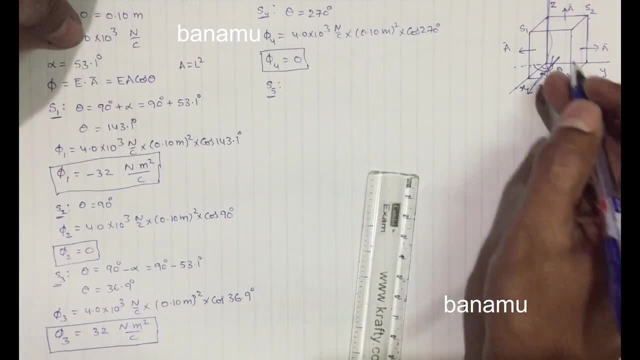 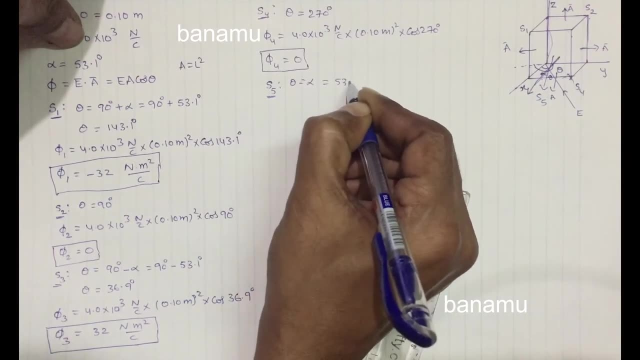 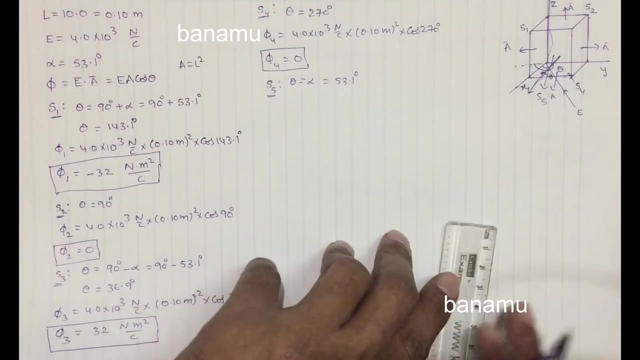 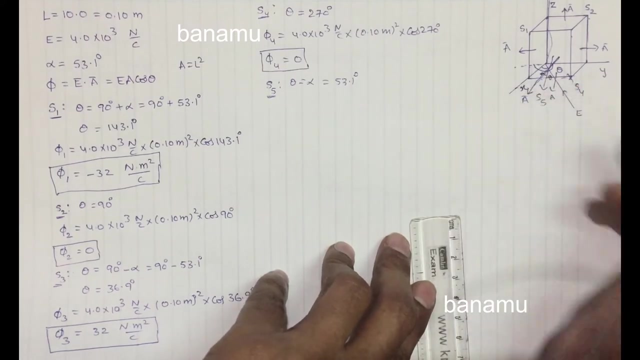 the angle between the unit normal vector to electric field is: theta is equal to alpha, that is equal to 53.1 degrees, because this is the front of the cube. so the electric, the unit normal vector is parallel to the unit normal vector is parallel to the x-axis, so the x-axis, the angle between the electric field to x-axis. 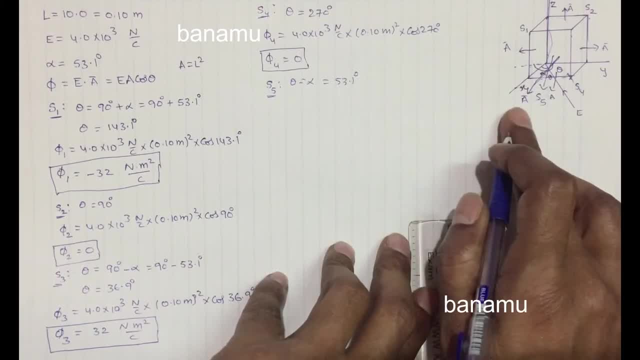 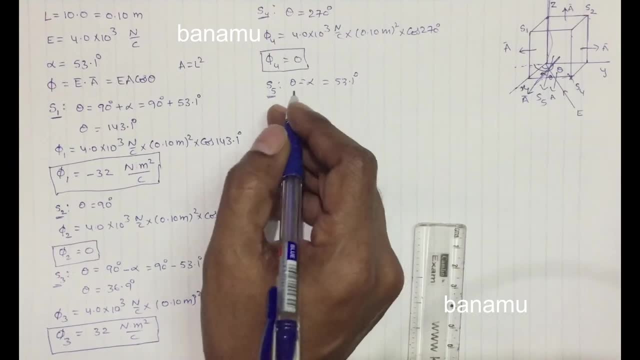 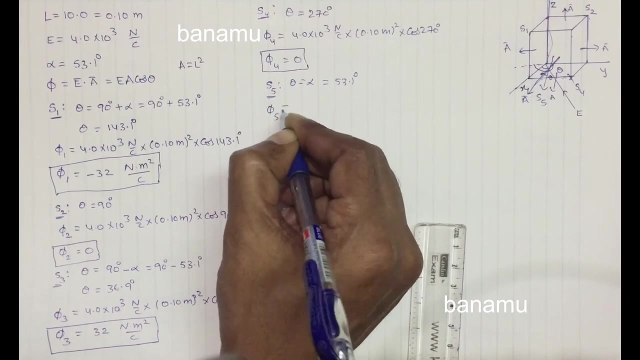 is the alpha, so the angle between the electric field to the unit normal vector is also alpha. so alpha is equal to 53.1 degrees. so the electric flux at that surface S5 is the 5 is equal to 55, is equal to the electric field, is the 4 into 10 to the power of. 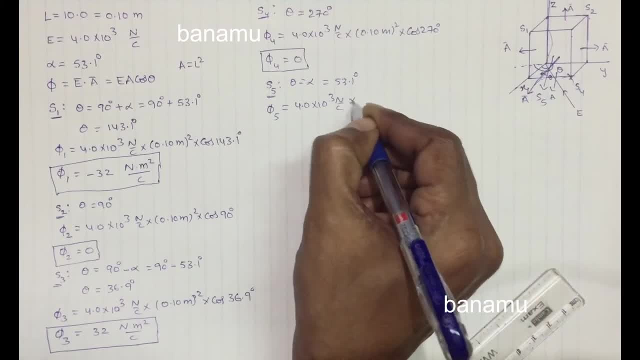 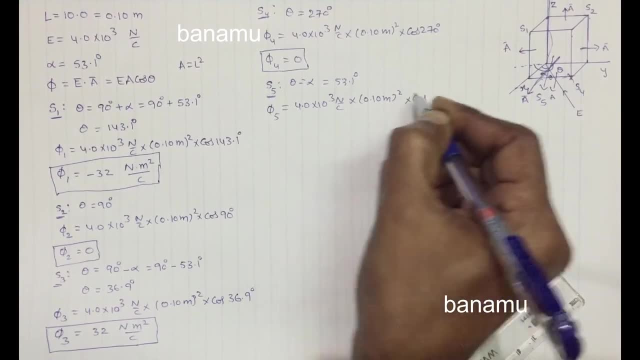 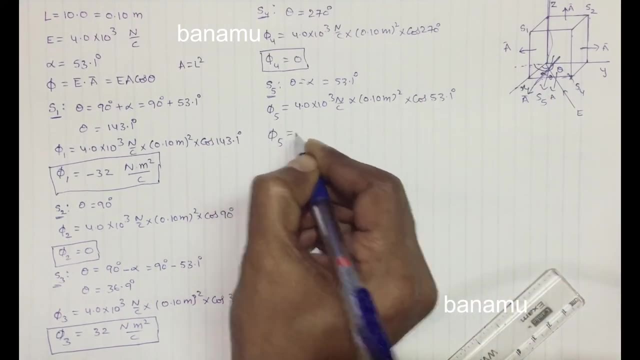 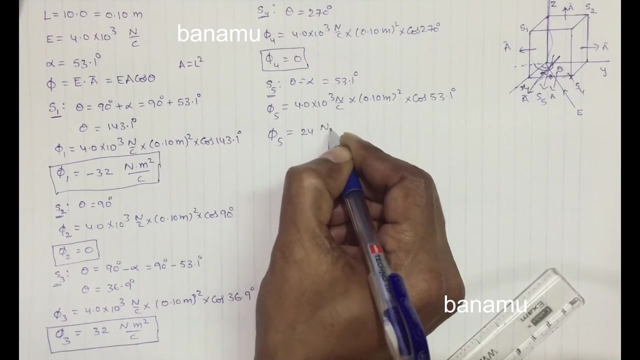 3 Newton per coulomb into the area is the 0.1 meter whole square into cos. the theta is the 53.1 degrees, so the electric flux at the surface S5 is 29.1 degrees. here we say 29.1 or exactly, and therefore minus 54larae by delta, x is 342. 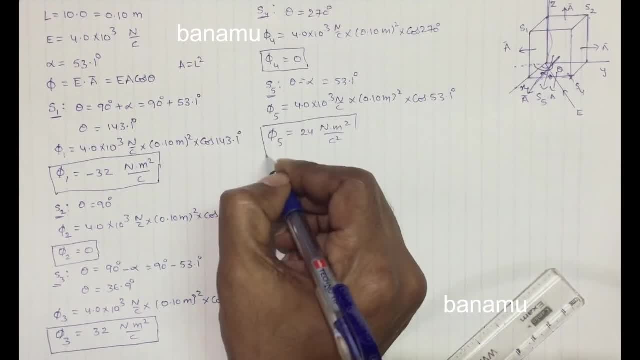 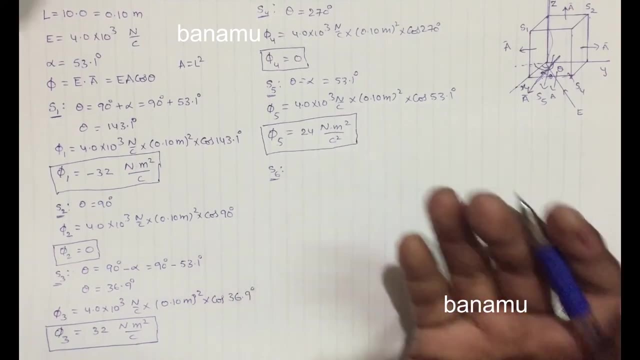 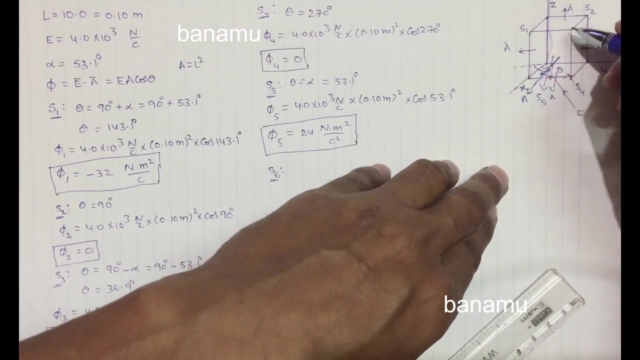 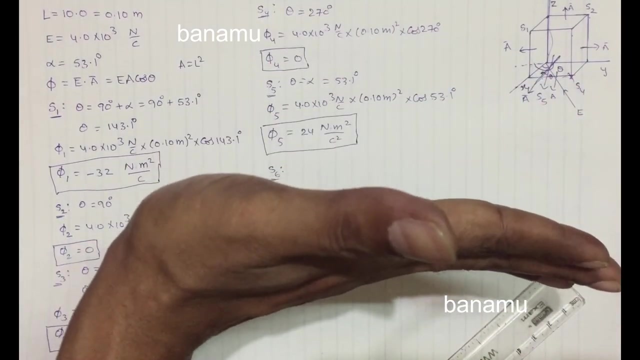 shorten forementeige, dan. so we get the moment. four Newton meter square per Coulombus Square. so this is the electric flux at the surface s5, a front of the cube, and the electric flux at the surface, yes, six, the electric flux at the cube. So this is the surface S6, this is the back side of the cube. So the unit normal vector. 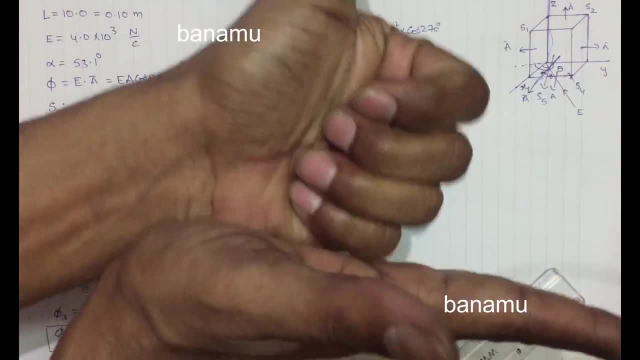 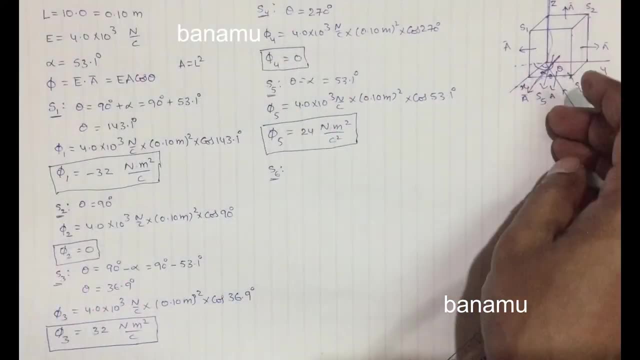 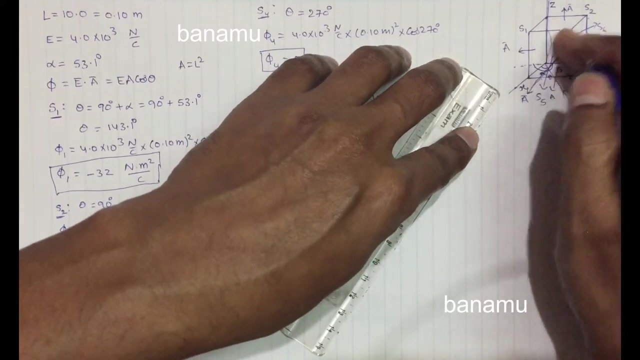 is perpendicular to the this surface. So the direction of the unit normal vector is the along the negative x axis. along the negative x axis. So the unit normal vector, this is the surface, this is a surface. S6, this is the back side of the cube and the unit normal vector is: 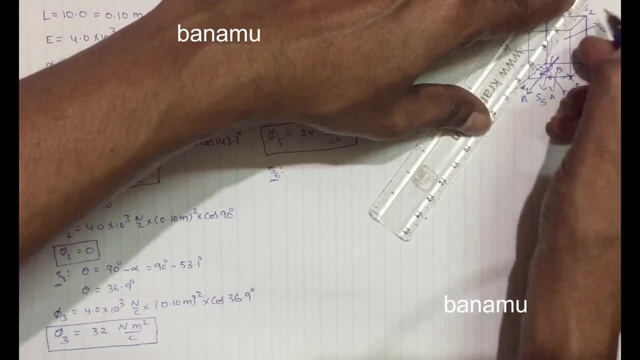 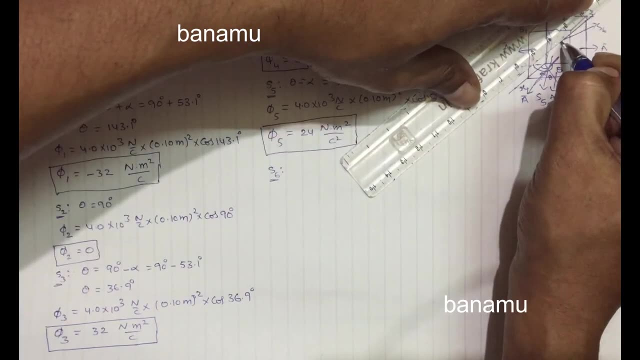 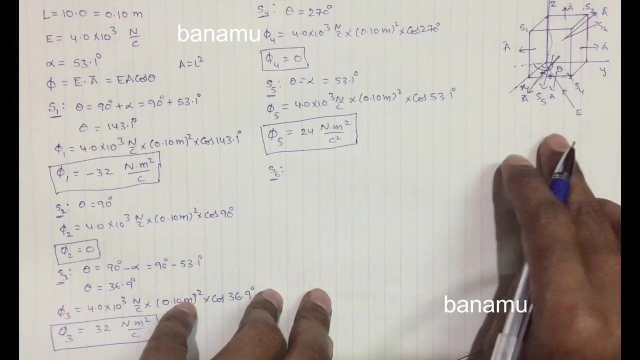 perpendicular to the x axis. So this is the unit normal vector. This is the perpendicular to the x axis, So this is the unit normal vector. a bar. So the angle between the unit normal vector to the electric field is: So the angle between the negative x axis to the electric field is: 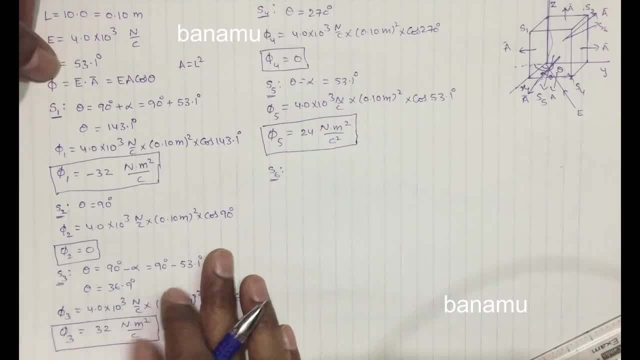 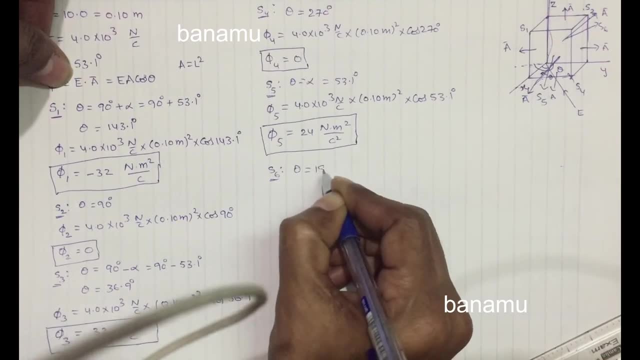 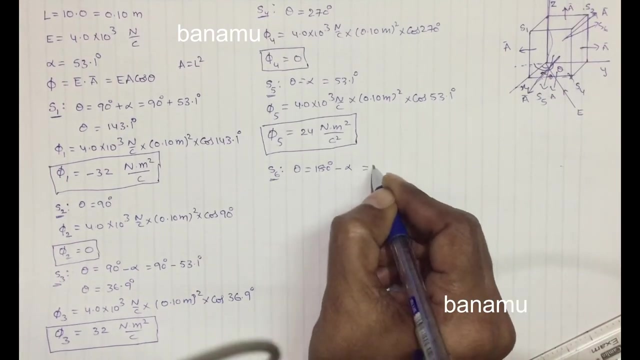 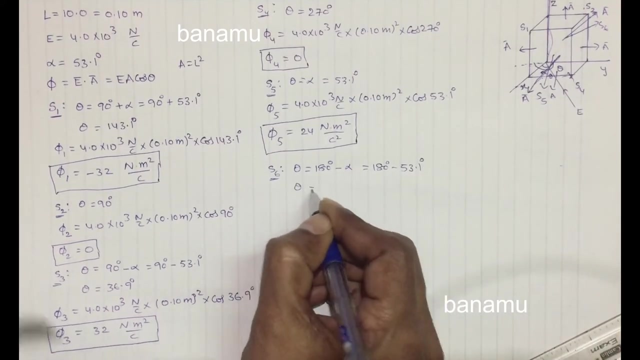 negative x axis to the electric field is: theta is equal to 180 degrees minus alpha. Theta is equal to 180 degrees minus alpha. That is equal to 180 degrees minus 53.1 degree. So theta is equal to 126.9 degrees. This is the angle between the unit normal vector to the electric field. 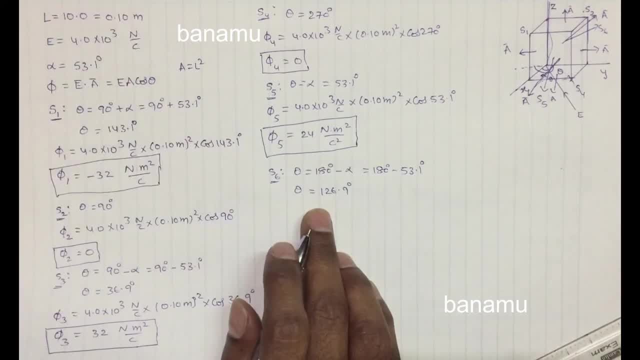 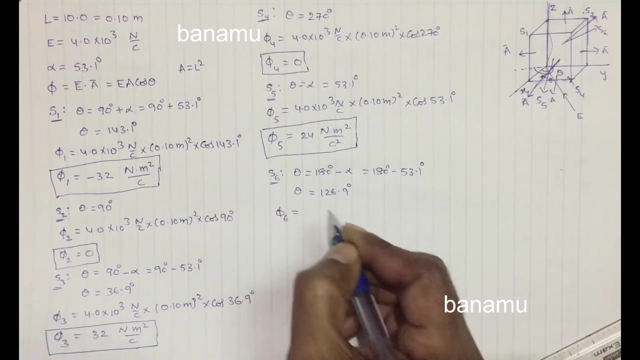 The electric field to surface S6.. Electric field to surface S6.. This is the angle between the electric field to unit normal vector. So the electric flux at the surface is 5, 6.. 5, 6 is the electric flux at the surface S6. So 5, 6 is equal to electric field, is the 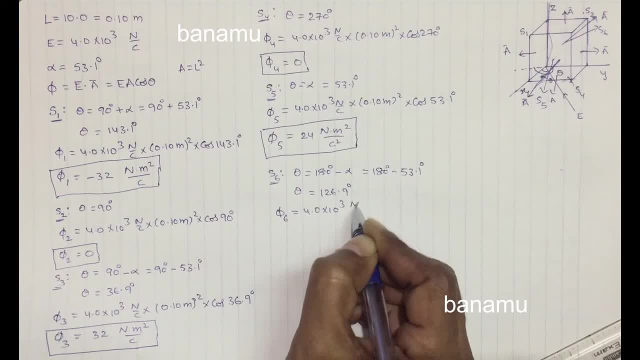 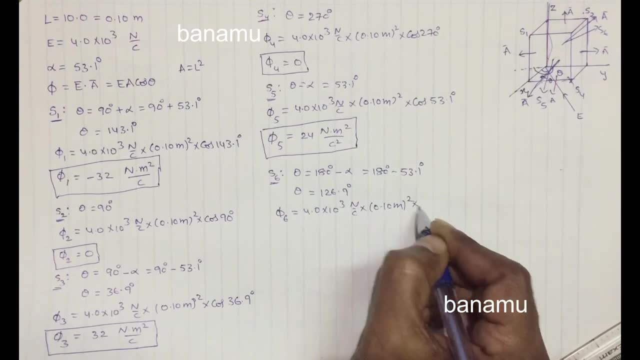 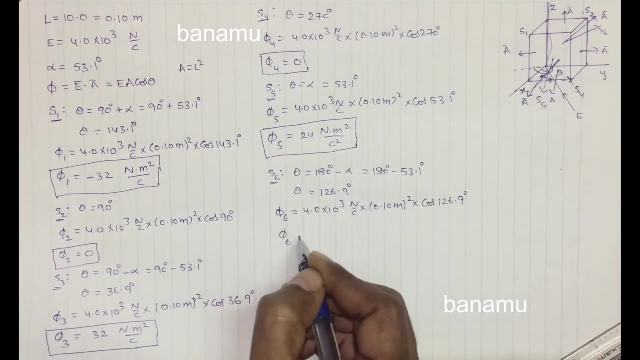 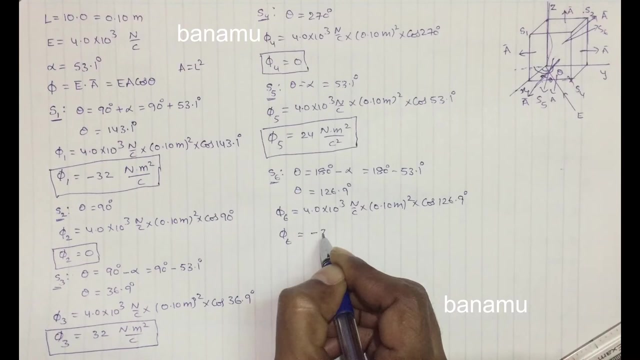 4 into 10 to the power of 3 Newton per coulomb into area is the 0.1 meter whole square into cos 126.9 degrees. So 5, 6 is equal to the electric field. The electric flux at the surface S6 is the minus 24 Newton meter square per coulomb. 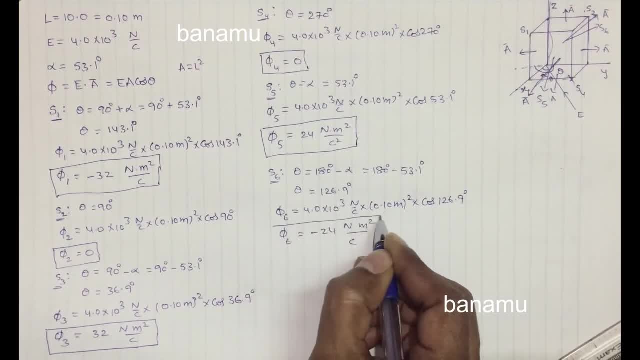 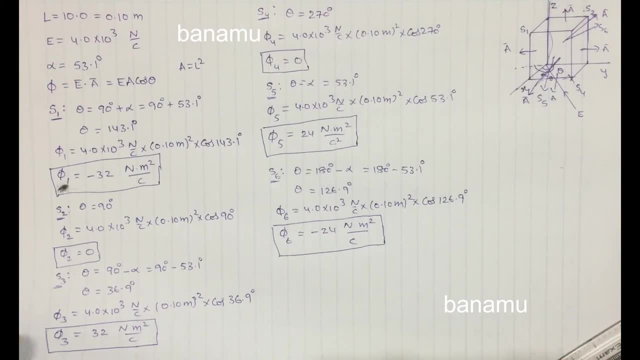 This is the electric flux at the surface. S6 are backside of the cube. This is the total electric flux. We can find the hot B. The hot B is the total electric flux in the cube. So the electric flux, the total electric.